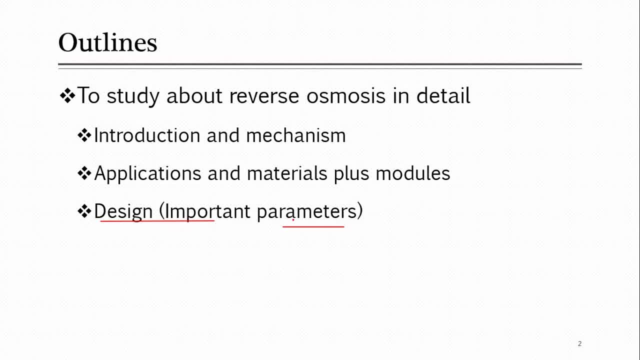 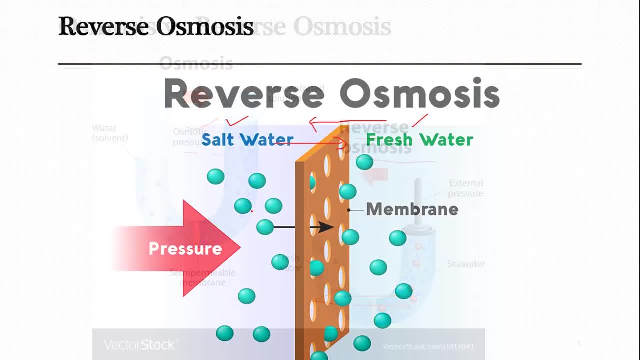 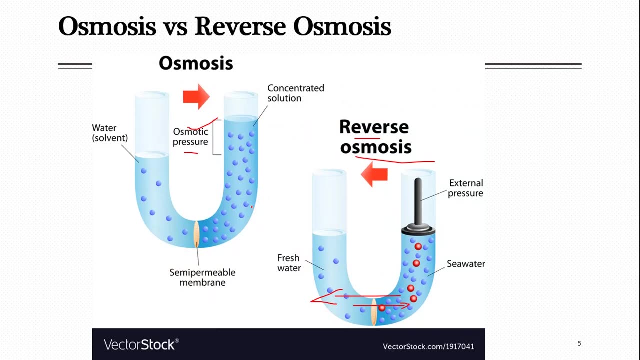 So quickly. I will just recall all the points which we have discussed yesterday that initially we studied osmosis and then we said that how it is related to reverse osmosis. So osmosis was traveling or movement of solvent through some semi-permeable membrane from 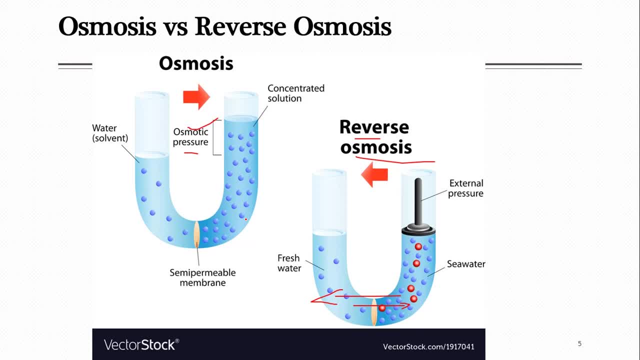 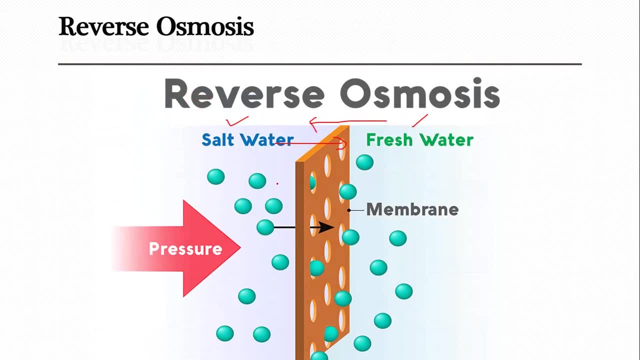 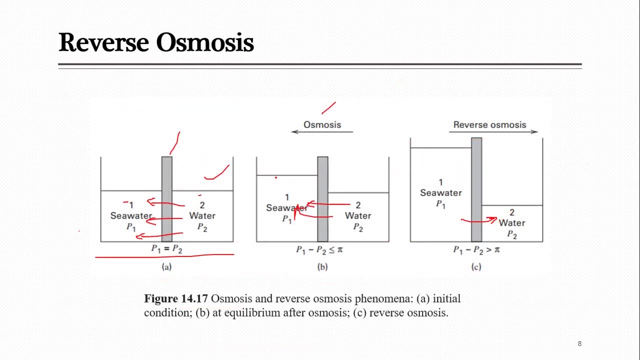 low solute to the high solute concentration and we said: if we apply any external force against this natural force, then we can reverse this phenomenon. that is called reverse osmosis, and reverse osmosis is actually based on your book. I mean, osmosis is not separation technique. 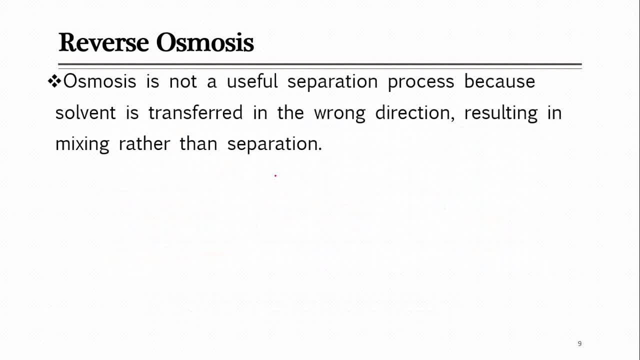 even it creates mixing. So we have to go in the reverse of this, and for that you have to apply higher pressure as compared to the pressure on the other side of the membrane, as well as osmotic pressure. You have to overcome all those pressure and then you can go for. 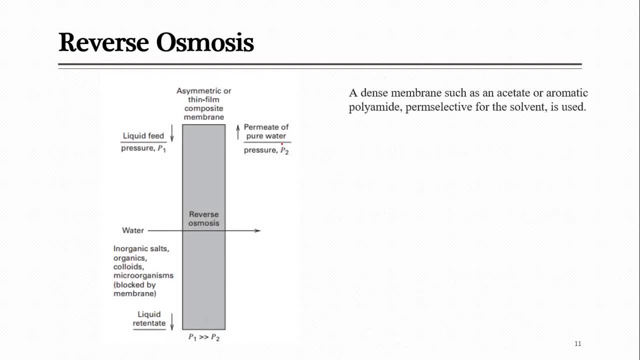 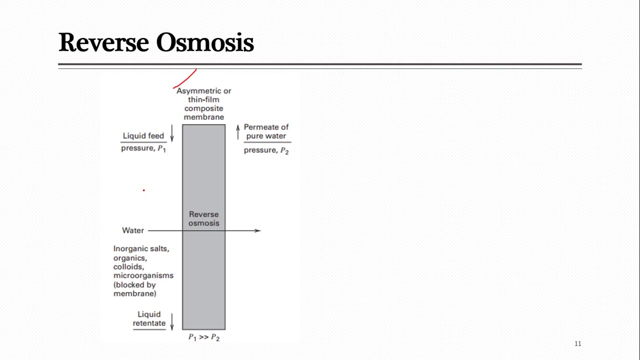 reverse osmosis. and then we said that most of the reverse osmosis membrane are asymmetric membrane. Why? Because you have a very high pressure on the both sides the membrane to for this phenomena you need some actually dense membrane for reverse osmosis and 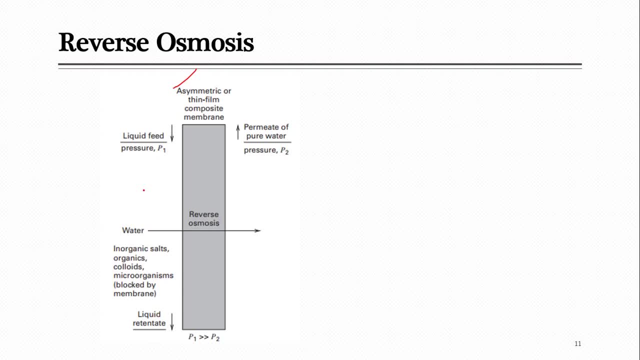 dense membrane. then dense membrane will be a like one sheet, very thin sheet that can't support very high pressure on both ends. so in order to avoid the rupturing of membrane, we make membrane as asymmetric membrane. its top layer is like dense membrane and below that there 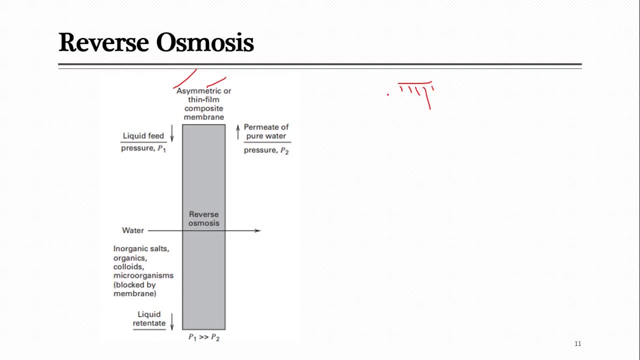 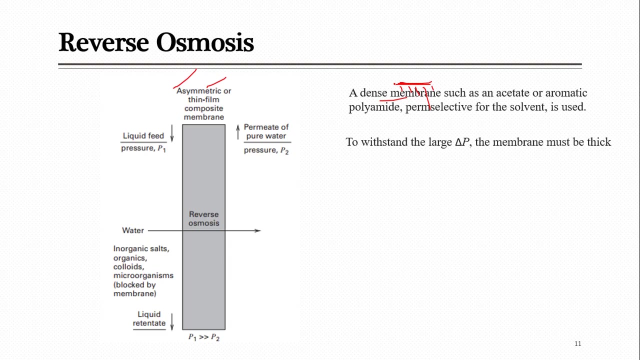 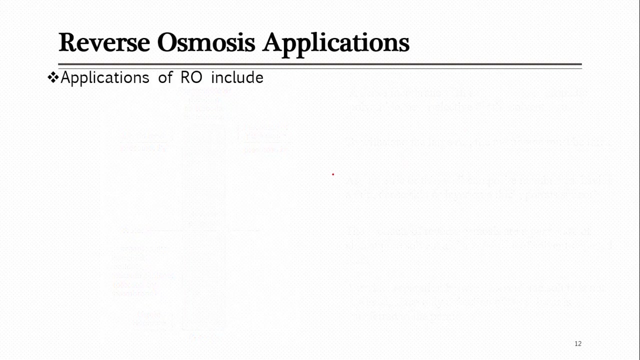 are porous membrane. micro and macro porous membrane can be used and they are just used for separation purpose, for support, sorry, not separation. they are used for supporting only the top layer, which is active layer and which makes separation. So in order to withstand this high pressure on the both sides of membrane, or transmembrane pressure, we use this and most of 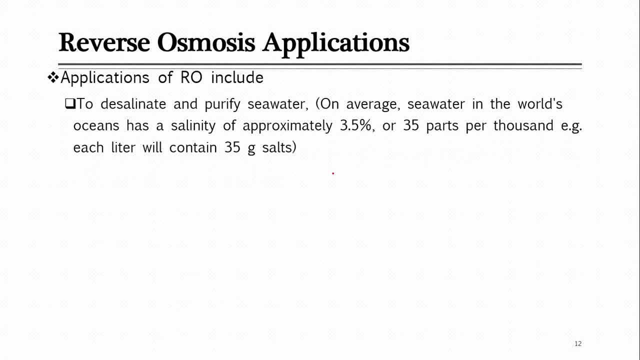 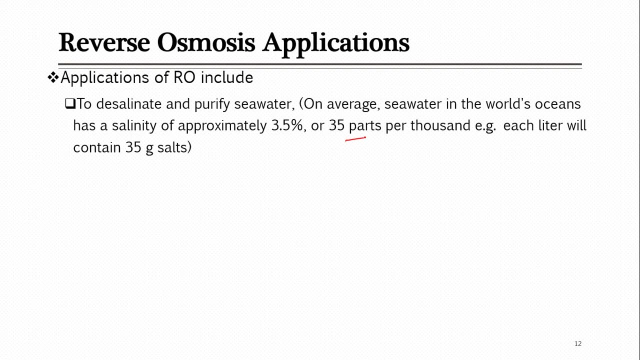 the time this RO are used, or reverse osmosis systems are used for cleaning of water. now here we have studied different type of water coming from sea that contain very high amount of solvent, even that's 3.5 percent or 35,000 ppm. and then 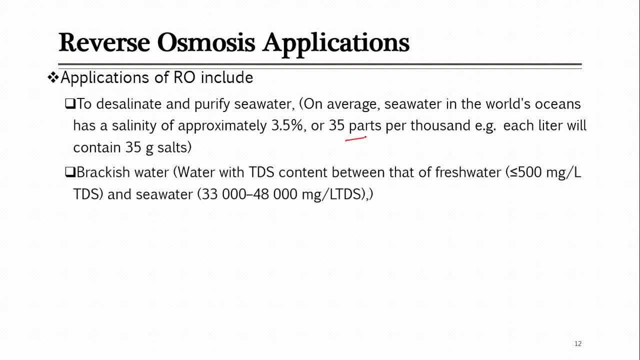 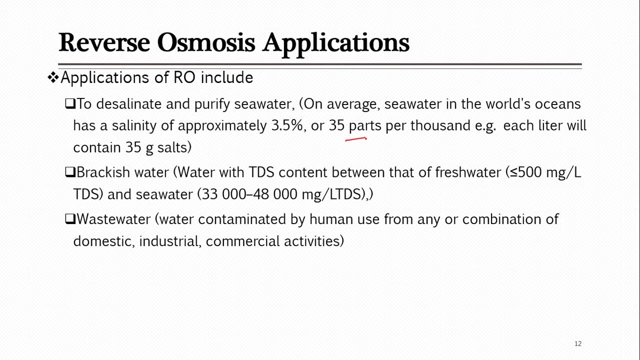 there is brackish water that has salinity or salt content between sea water and fresh water, and fresh water actually contain 500 ppm dissolved solids. and then there is wastewater. wastewater is actually water coming from all human mean which is contaminated with various pollutants due to human activities. those include 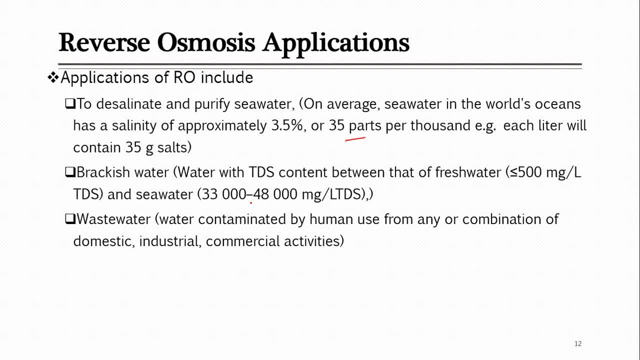 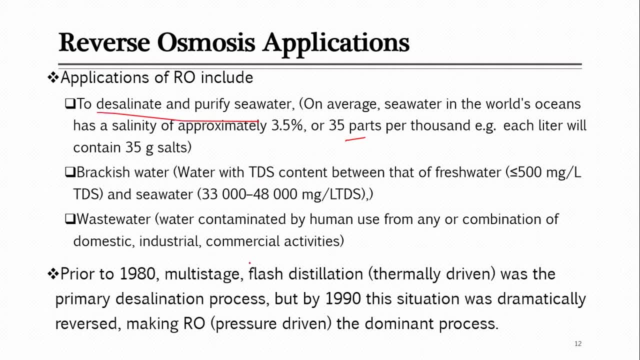 industrial, domestic, mean, agricultural, cultural and all commercial activities. and then we said that actually before 1980, mainly for desalination purpose, flash distillation was used. and that's flash distillation- actually involve high temperature, you have to heat the water and you boil. water and salt are left on the surface of the equipment in which that water was contained. and 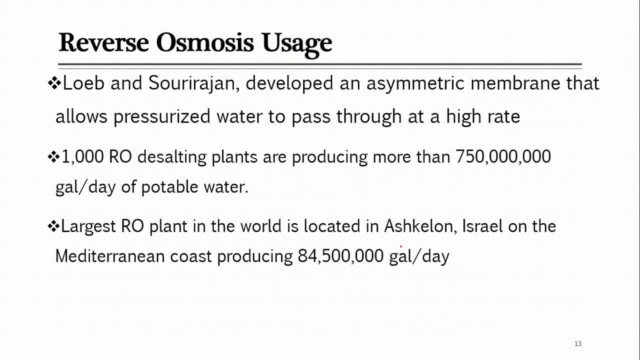 then water which is boiled is condensed. that was highly expensive technique because it involve large amount of heat, so that was replaced with the efficient membranes in 1990 and recently. a lot of plants are used in the world. around thousand plants are used and they are producing daily 750. 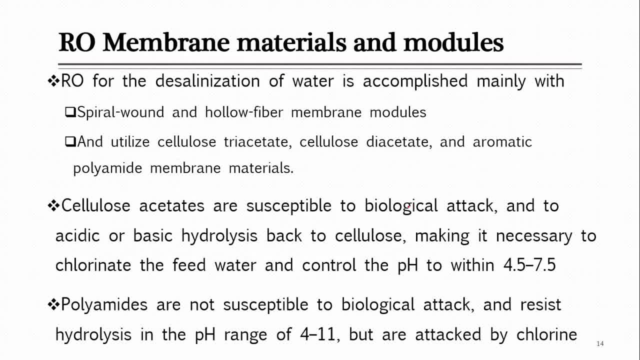 million gallon per day of potable water. Then we looked at that majorly. spiral wound and hollow fiber membrane modules are used because they can withstand high pressures as well. there are cellulose acetate based and polyamide based membranes are used for these separation, although both membranes suffer from some problem. but they can be overcome by pre treating the 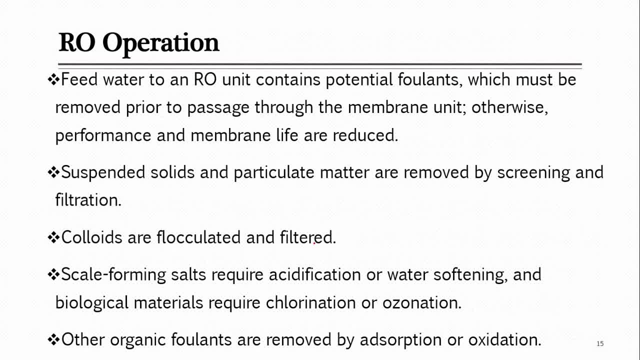 water and then, as we said, water contain a lot of impurities. there are not only salts which can be rejected with the reverse osmosis membrane, So some of those can be even separated before bringing it to the membrane. and why we separate all this stuff here. we discussed that you can use either various type of other porous membrane like micro, ultra and nano filtration membrane to remove some of those contaminants, and sometime you can also use various other processes like flocculation filtration. there is ozonation, chlorination, these oxidation and adsorption. these are various other pretreatments which are used before bringing it to the membrane. 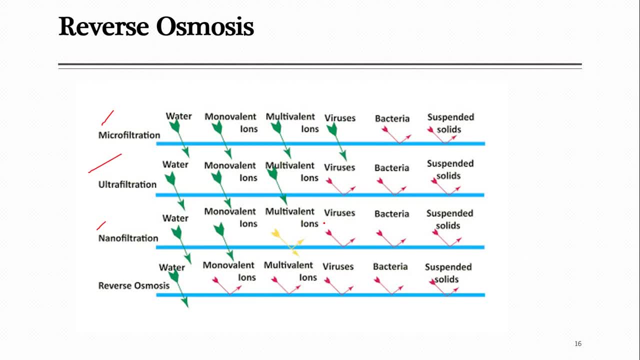 So these are all the step project activity which is really important. no, of course you have been taking some lot, but the essential of the�� super integration required for the wringing like water, for final touch or for final, I mean removal of monovolent ion. actually, these monovolent ions, for example, diplomatically A CL, KCL, the majorly is NA Tab. 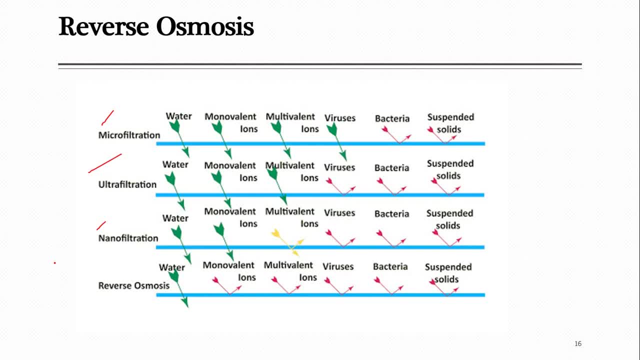 As if I took all without a doubt to that major questioncy: water. ah so and 36河 situations is not used for desalination plants, as I've been. it can be used for various other water treatment plants, but mainly for desalination project. of this, I'm talking about the anyway, because even products and so on can be performed against all those contaminants lower. it contains del focusing, so it can also remove aical chromium. gentlemen, Richmond glass can really help your body. an hashtags. 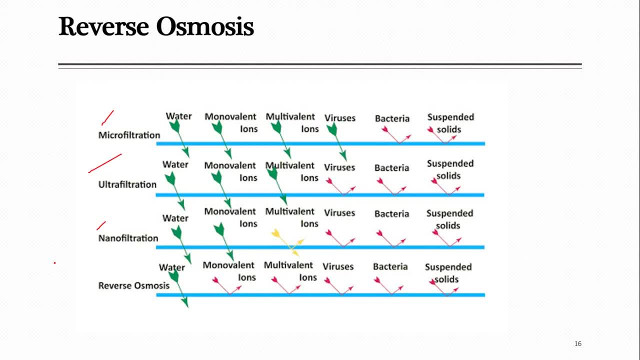 this. I am talking about these monovalent ions. So these monovalent ions cannot be effectively treated or separated by using any other technique, like these porous membrane or even adsorption and all other technique which we have seen. ozonation mean chlorination. those techniques 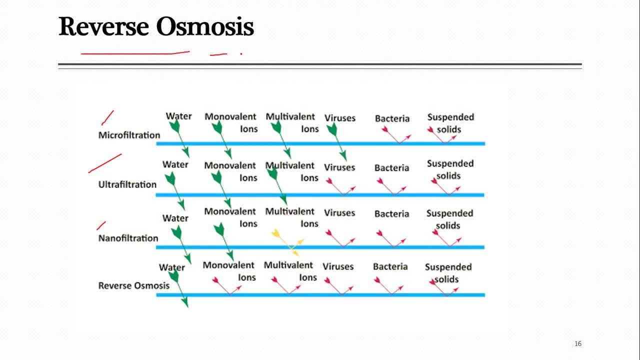 So that is the only solution. reverse osmosis membrane or mean distillation by heating the water and precipitating or separating the salts. So, as we said, that distillation is more expensive. So, due to this, we go for reverse osmosis and in this, reverse osmosis. 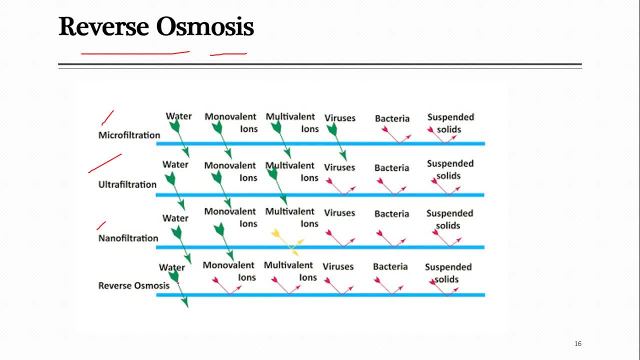 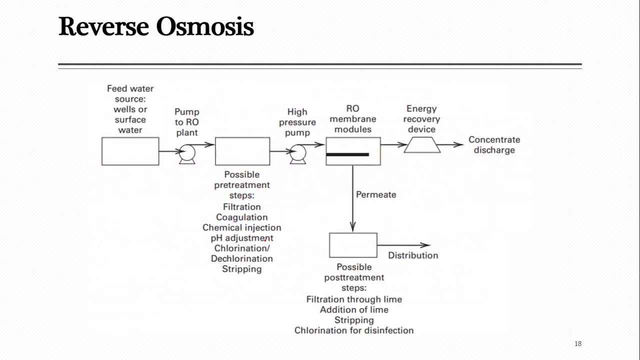 final stage only. I mean these membrane are dense membrane, which allow only water to pass through, and monovalent ion, which are solid. they are just separated here. So we also discussed this system. that mean that somehow the same stuff but in the form of like PFD, in which you can see that feed water tank, from that it is pumped to some. 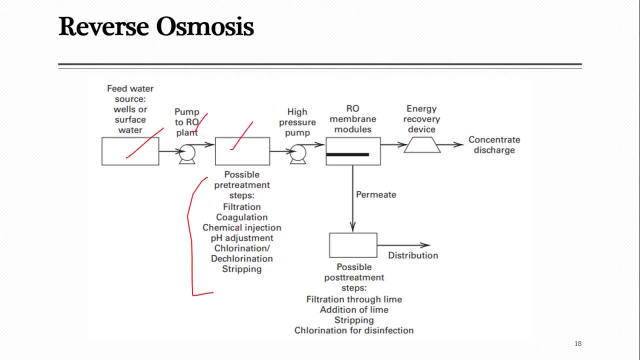 pretreatment unit and that can be more than one pretreatment unit, as shown here. So various it is not necessary always to have all these units, but sometime you can have like 3, 4 or 2 or 3 of these units most of the time and then you go for high pressure. 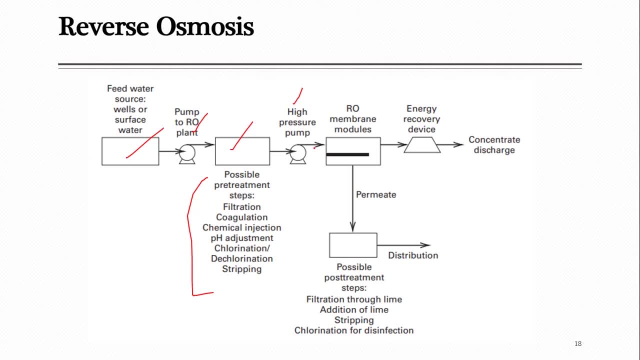 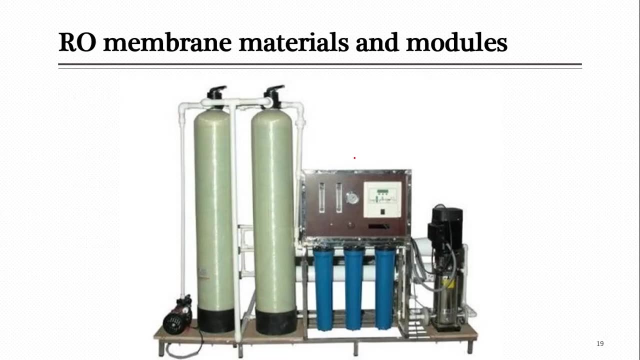 pump and that is high pressure is generated, actually to mean to just get permeate or high amount of permeate through the membrane. And with this I mean we finished last lecture up to here and at the end I advise you to just go through the text book. there he has explained the use of actually reverse osmosis. 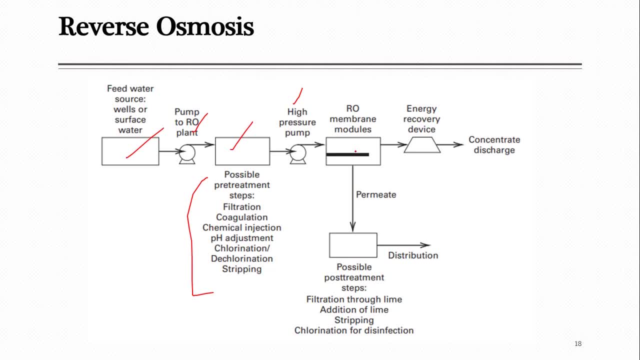 membrane for various treatment plants like textile industries and many other chemical industries for waste water treatment. So just quickly go through them and actually you should have the idea that where reverse osmosis can be used, I mean for desalination- definitely it is being used for various industries where it can be used. 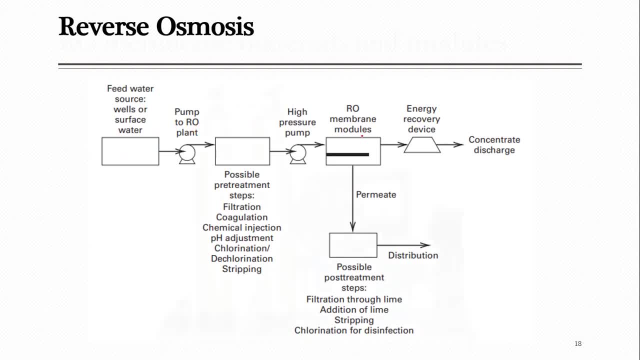 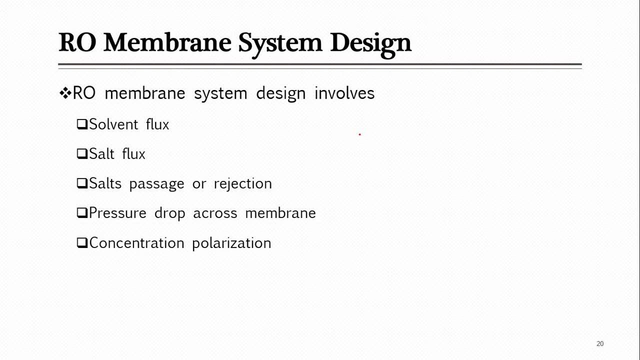 So many example he has provided. I think 8 to 10 examples are provided in your text, kind of the just look at them. So let us start with today's topic, that is, reverse osmosis membrane system design. as I finished yesterday my lecture at this point. So I told you that there are various factors. 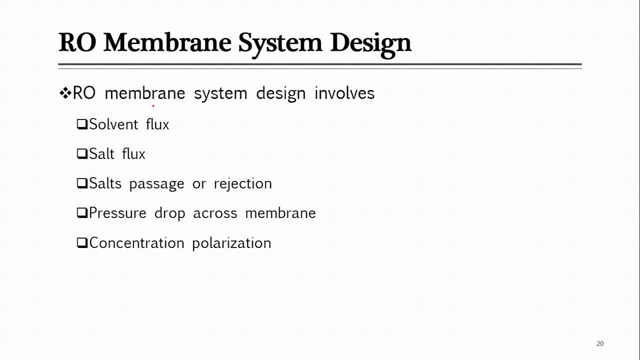 that you have to keep in mind or various calculation which you have to make while when you are going for like designing of these system or membrane system. So those calculation involve solvent flux. solvent mean majorly it will be. if we are using for, For desalination purpose, it will be water. otherwise, if you are using membrane for any 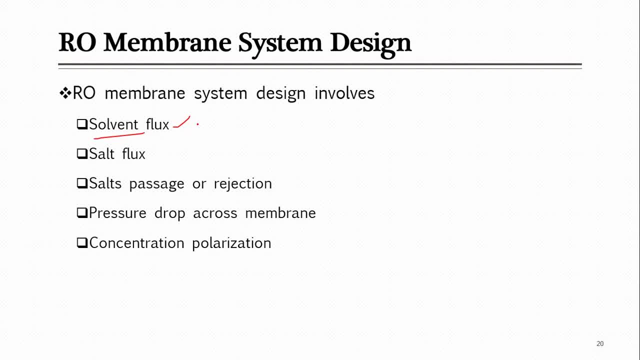 other separation, these RO membrane. So then the solvent, that species with just permeate through the membrane and is obtained as a permeate, that solvent, Its flux calculation mean how much amount is passed, or what is its flow rate per unit area, Its calculation? 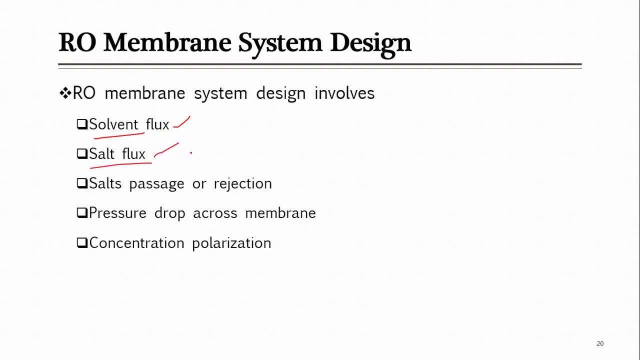 then there is salt. flux is some time. as I told you, mainly reverse osmosis membrane are being used. So these are the major calculation which we are going to look. here are stuff that deals with the solvent, like it will be water and salt which are present in the water mean as: 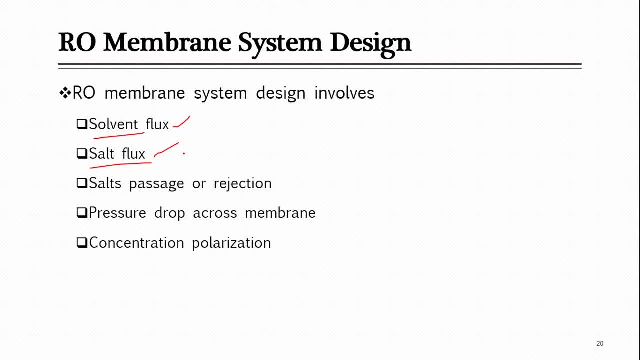 I told you in last lecture that these membrane are not only 100 percent selective for water, they can also allow other contaminants to pass through, but they pass like in very small amount. Like salt can also pass through that membrane, but they are passed in very small amount. 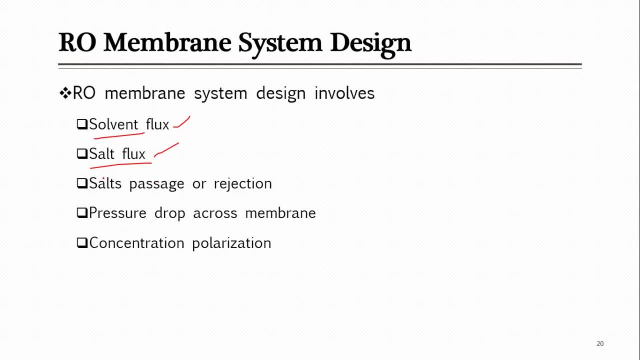 And this salt flux, calculation, that how much salts were? I mean pass through the membrane, and then this salt. passage or rejection mean. these are the factor which are also calculated or used in calculation. So rejection mean how much were rejected, and passage how much pass through this membrane along with water or the solvent. Then pressure drop across. 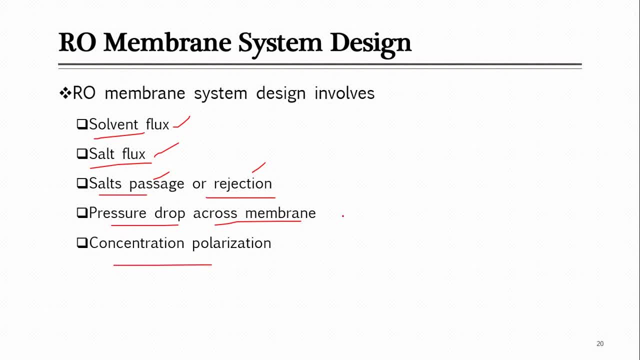 these membrane. that is also important parameter. And then finally there is concentration, polarization. So let us look at them one by one here I will go through them. major formulas and their calculation. we will not go for the derivation mainly. there are few steps which are actually missed, but major steps are given here for calculation. 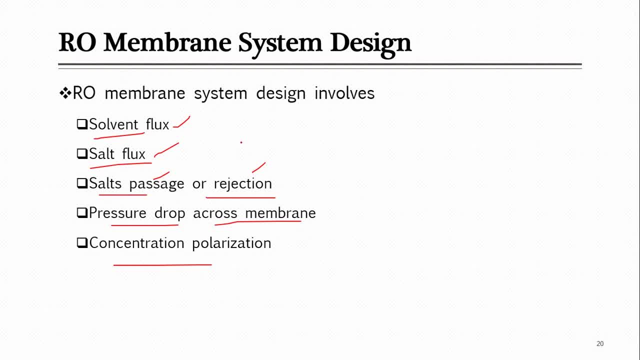 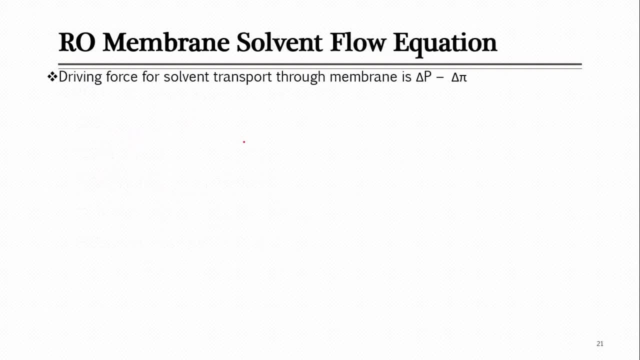 purpose. So at least you should know how to use this formulas and what are the terminologies involved in these formulas. If you recall, few days back when we started with the membrane separation there, we studied that actually permeance, or I mean this passage or flow of solvent through the membrane depends. 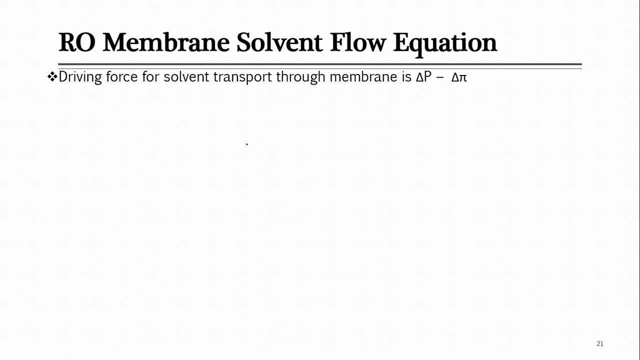 on two parameter, that was permeance, and permeance was permeability divided by the thickness multiplied by driving force. So here, majorly for this system, when you are using it for desalination purpose, mainly the major transport or force, here driving force is actually pressure. 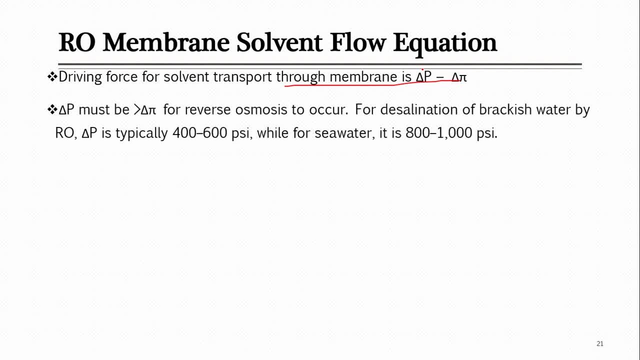 difference across the membrane and that is delta P here. pressure difference, as we said that this is transmembrane pressure, suppose it was two cells, So there was a membrane on across this there is P1 minus P2.. So if you just take this difference, suppose P2 side. 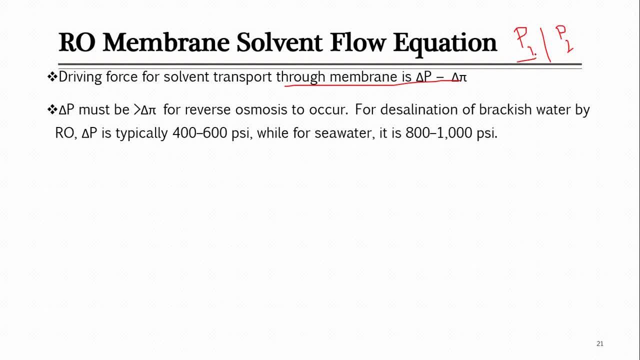 is the pure solvent or pure water, and P1 is the solute, So solution side. so here P1 minus P2 is the main difference in pressure and we said that. I mean then there is osmotic pressure on both side if this is pure solvent. on this, 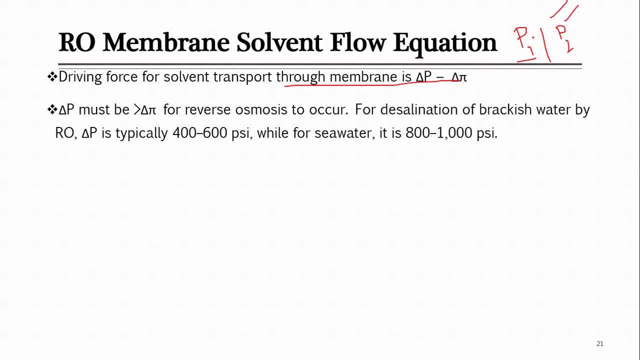 side there will be, pi will be 0, as talked in last lecture, and here on this side definitely it is solution- salt will be there. So there will be something, some value of this osmotic pressure pi. So here delta P must be greater than delta pi for reverse osmosis to occur. 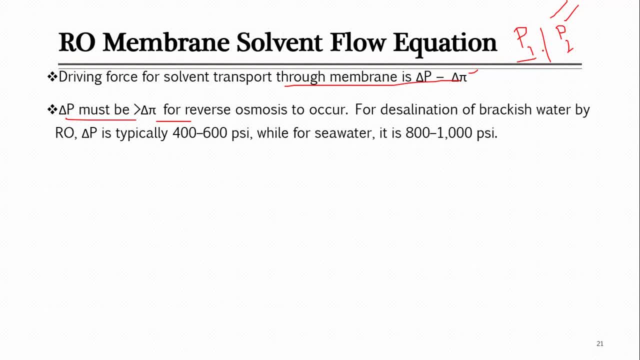 yesterday. Also, we described- discuss this point at this- that pressure I mean here should be higher. P1 should be sufficiently higher for this passage of solvent through the membrane and for this reverse osmosis to take place For desalination purpose when you look at brackish water. so this pressure actually across. 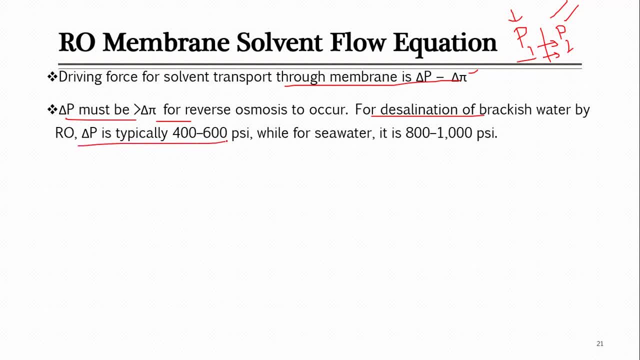 the membrane, or delta P value, is between 400 to 600 psi as well. for sea water it is 800 to 1000 psi. this is a huge pressure which you have to apply across the membrane, Like suppose you are getting water on this side of maybe just at normal pressure of 1. 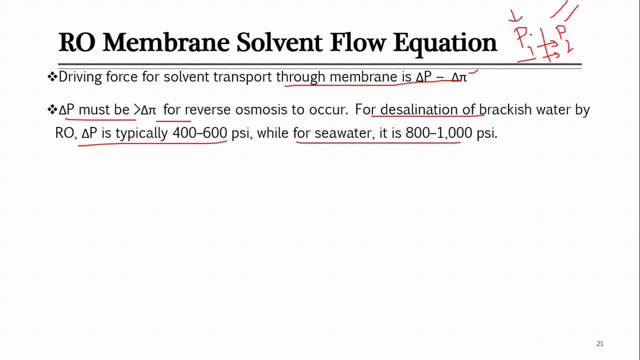 atm or 14.7 psi. so on the other end it will be very high pressure, and most of the time here if I talk about in atmospheric pressure, so it is like somehow it will be around 20 to 30, I think, psi, and the other end it is usually 2 to 3 psi. 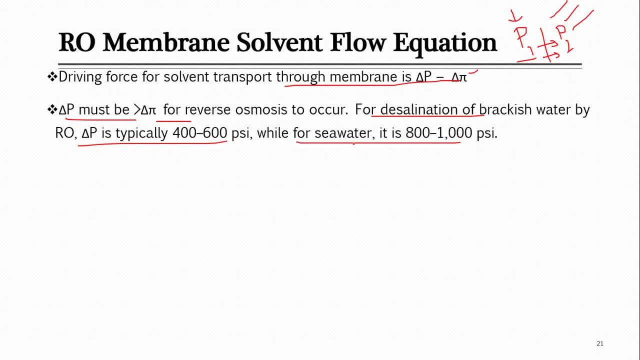 So just another thing in your book is also provided related to this. he has provided various exact example for this- that if you are looking for some separation of brackish water or sea water, so how much should be pressure and how much salt are recovered and how much permeate? 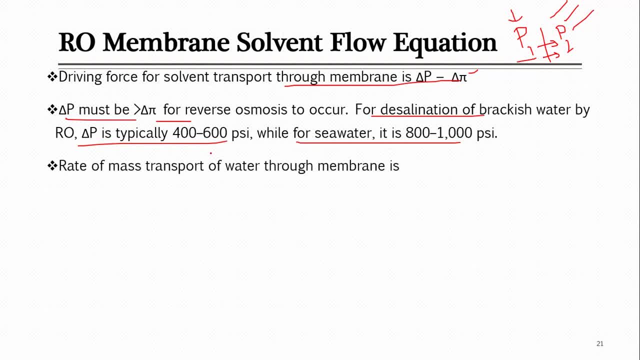 you get just go through that for your information. Mean, that is also available along with the examples of main membrane, RO membrane for various industrial plants. Thank you, So that is on the same page. So, rate of mass transfer of membrane, this water solvent or water through the membrane. 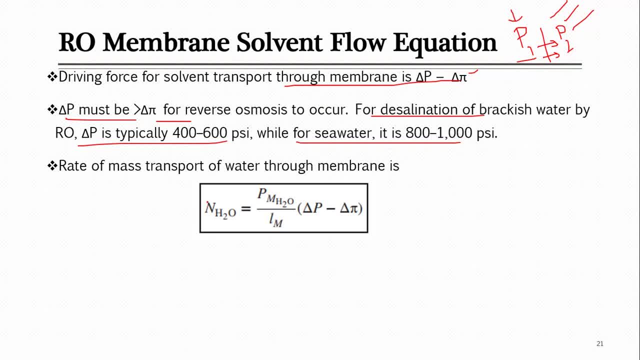 that can be calculated. actually, the solvent flow that can be calculated by using the same equation which I just started with. I was telling you that that was mean flow of or number of moles of some fluid solvent passing through the membrane is equal to. this terminology was called as permeance. 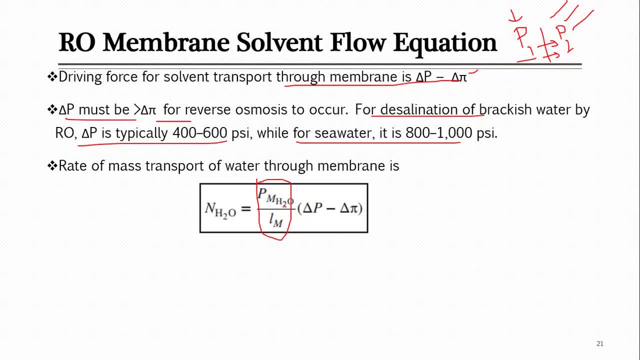 That is, permeability of that component through the membrane. that component is here water, because we are talking about water. so it this component, this will be in a molar flow rate of the water and this will be like somehow: permeability of water through the membrane and for membrane. and then there is thickness of membrane and this is driving force delta. 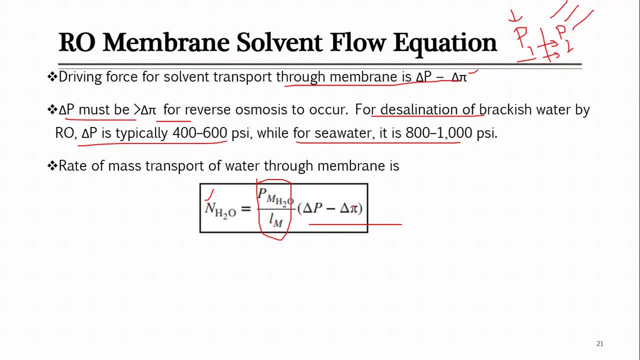 p minus delta pi. So there is, I think, derivation of this equation in your book, But no need to go through all the equations, No need to go through all that, just remember this formula and use it. So here, delta p is actually indicates pressure: hydraulic pressure difference. 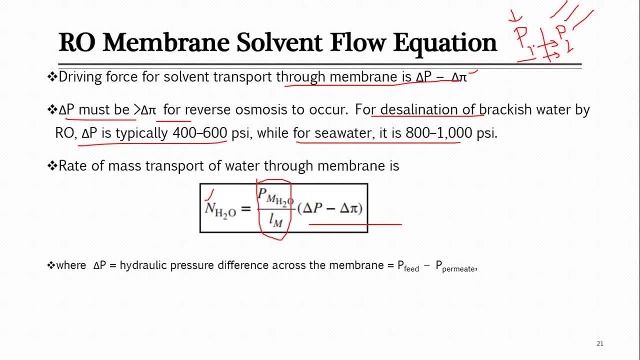 So pressure on the feed side and permeate side, So that can be measured and we will have it like delta p which can be calculated. Then there is osmotic pressure. So osmotic pressure, that is mean again delta pi. So one side is feed side, this from where feed is entering, this he is calling as feed side. 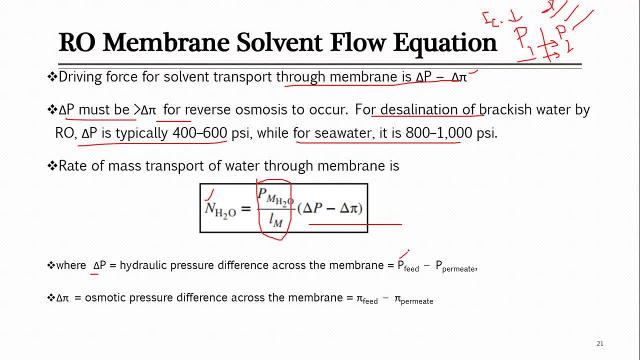 and other is permeate side, from where permeate is entering. So same for pressure on the feed side minus pressure on permeate side, and this osmotic pressure on feed side minus osmotic pressure on permeate side, that is delta pi. Then there is, as I told you, this mean permeability. this is the membrane property and most of 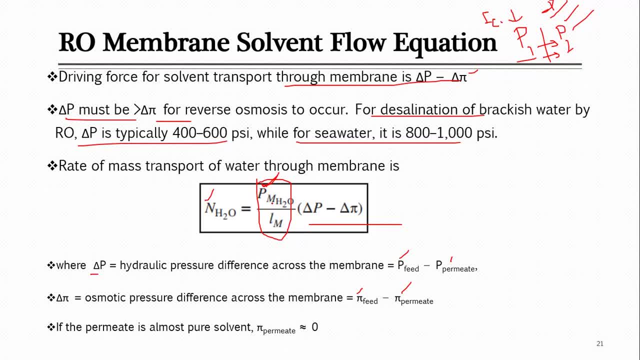 the time we get it from experimental data that is provided, usually based on interaction of any component, like here water, with the membrane material and thickness, and most of the time So in your book this is given as a complete permeance value, that is, permeability divided. 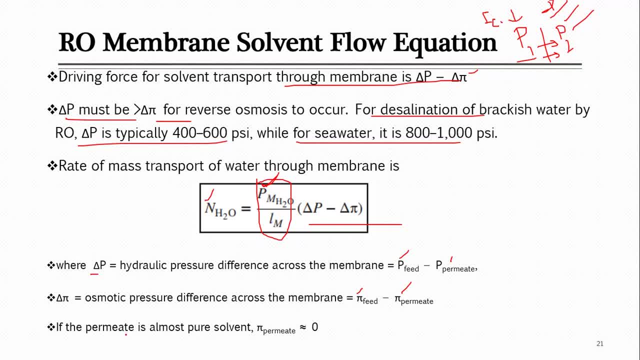 by thickness that is given as a permeance. Here I mean this: if you have to calculate osmotic pressure, So that can that? that can be calculated like: suppose if permeate side, on permeate side it is pure solvent, and you know when it is pure solvent there will be. no, there will be. 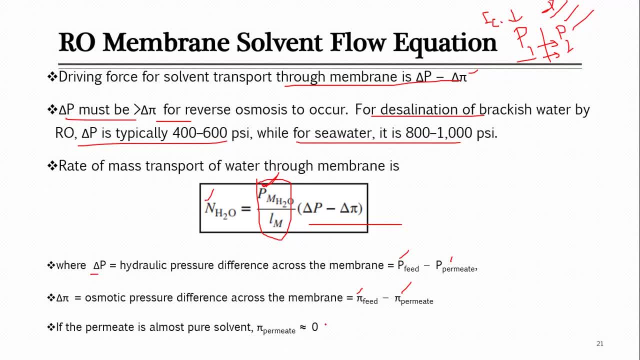 no like salt or no solute there. So as yesterday we saw, So yesterday we saw that journal formula which can be used for this: that was equal to pi, is equal to mrt and m is molarity, that is number of moles of the salute. and when 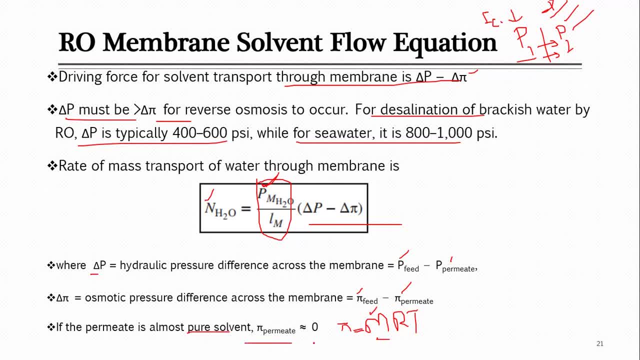 there is no salute pure solvent then it will be like 0. due to this he said that pi of permeate- osmotic pressure of permeate- then in this specific case of pure solvent, will be equal to 0. So here in your text, there is one equation provided for sea water, one correlation provided. 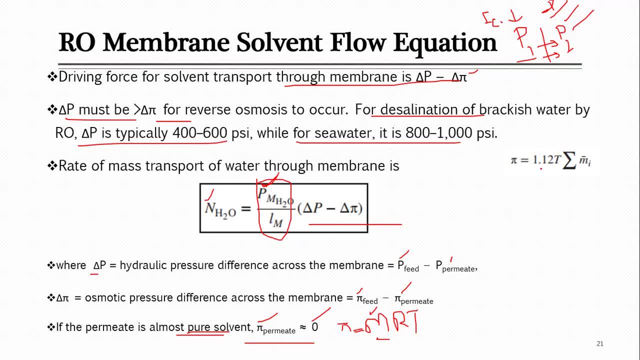 for seawater calculation because that is dependent on many factors here. So they have provided, because seawater, as we have seen yesterday, that seawater salinity varies. So that is one correlation given here in the book for seawater osmotic pressure calculation, like 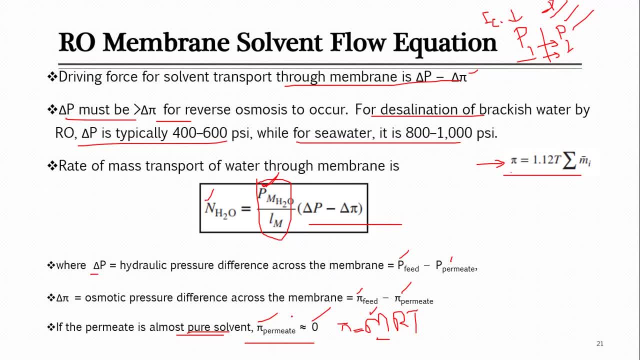 suppose you are, given that seawater is entering to the membrane on feed side, you can calculate this pi as well. you can use this same for the permeate side as well as for feed side. So that is equal to 1.12 t into summation of. I mean molarity of all components. So 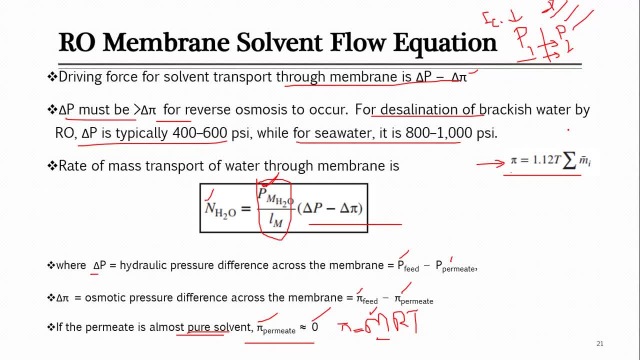 overall. suppose there is one component, for example water contains only NaCl, So it will be only molarity of that NaCl. and then, if it is like more than one component, for example there is also KCl, So it will be some of the molarity of that. 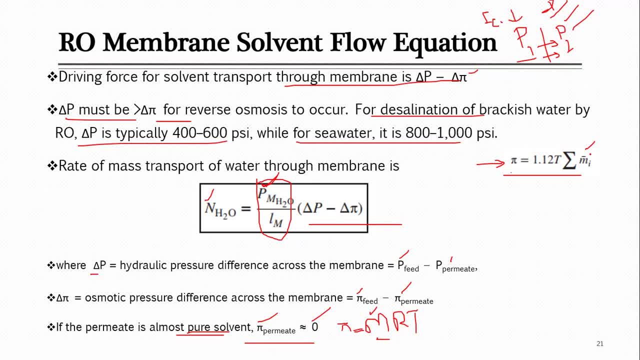 component. and one thing remember here: when you have to use this formula of molarity, this is some of the molarity. suppose you have NaCl, So when it get dissolve inside water, So what will happen? I mean, it is broken down into two ions like Na plus and Cl negative. 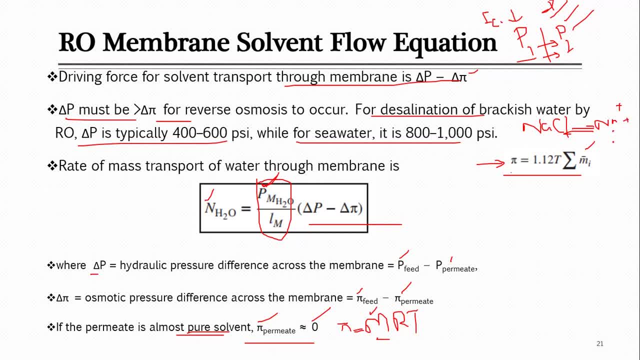 you know this just split into its ion Na plus and Cl negative. So actually we will calculate molarity of Na plus molarity of Cl. So this is the part of the compound. it is based on each individual component. So if 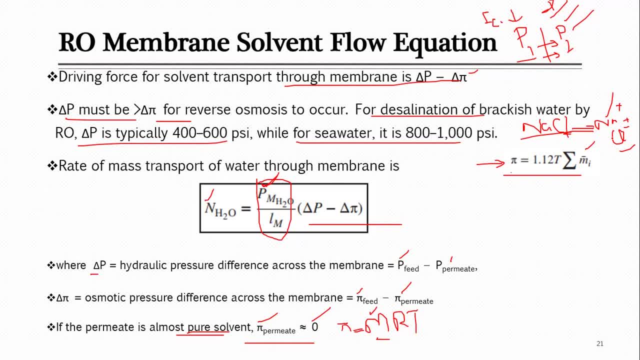 Na and Cl. So overall I mean just they are same, like one mole of this is produced and one mole of this. So overall, if we calculate the molarity of one, we can just add it up to get the molarity of both. but if also there is like something KCl, So there will be one. 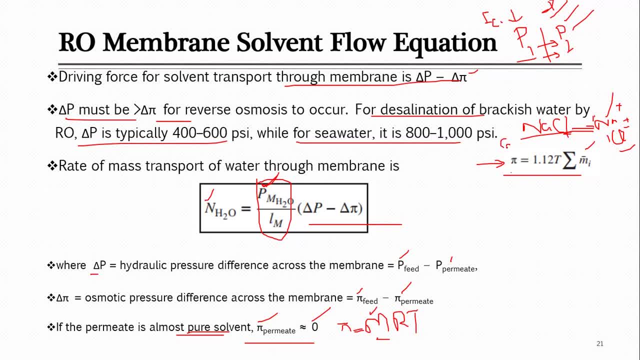 K and one Cl- again same, but for example you have CaCl2.. So in this case number of mole of Cl2 are double as compared to the Cl2. So it is molarity when you have to calculate, for example for calcium and for calorene. 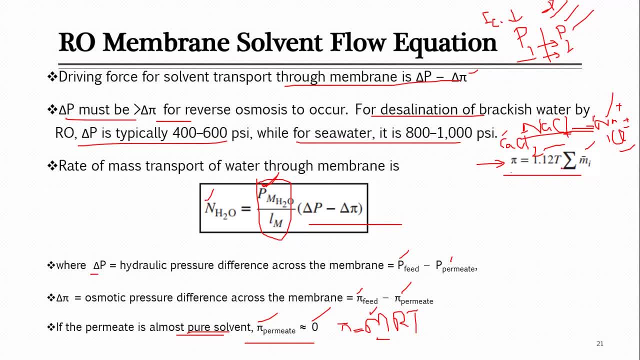 So then you have to add them up. So overall, this equation can be used for calculating osmotic pressure across them on the both sides of membrane, on feed side as well as permeate side, and we will use this in one of the problem today we have to solve at the end of this. 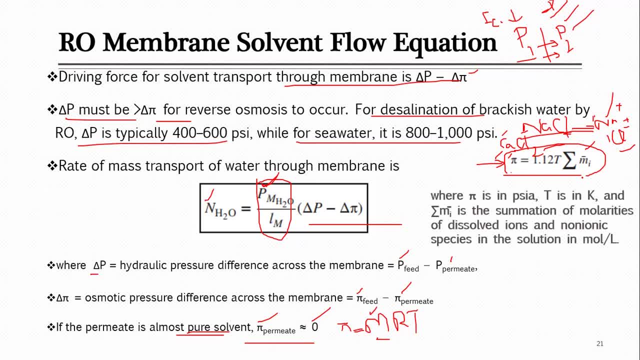 lecture. So you can. you see the utilization of this equation. So here, but the few things are necessarily to remember when you are using this equation. here, I mean, units are very important- pi, as per this overall correlation at the end of the day, Here what we did actually. you can see that r was replaced. you do not have to. 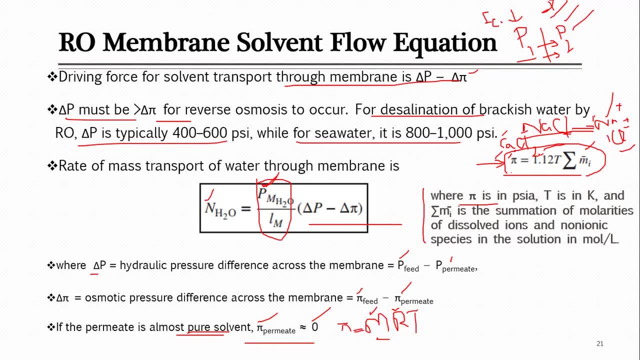 put, you do not need to worry about the values of r and this correlation may be was derived in order to avoid this problem of r, because some time you can get confused with the units and that stuff mean value of r is already, I mean, inserted in the equation and this final correlation is given. 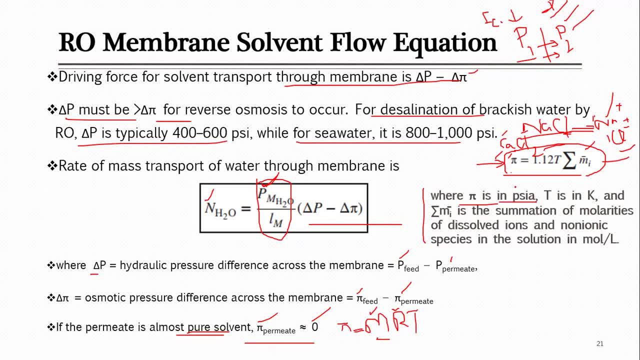 which you can use. So pi is in psi, pound per square inch, absolute, and t is in kelvin. here, when you have to use this equation, use t in kelvin. and this mean m i sum of molarity of all components, that is the summation of molarity of dissolved iron and non-ionic species in. 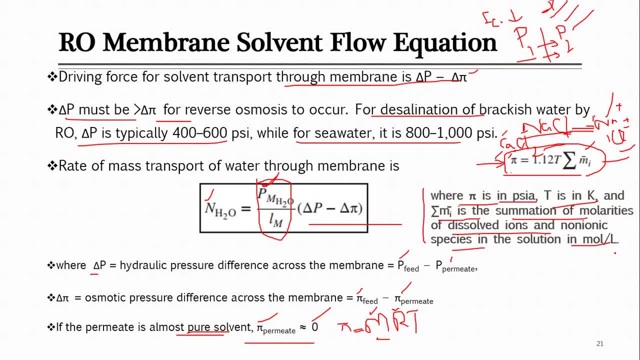 mol per liter. Suppose there are ions and sometimes there can be impurities which are even non-ionic, but they are available inside the system, So they can also. they will also be calculated and this final unit of molarity is actually in mol per liter, For example. 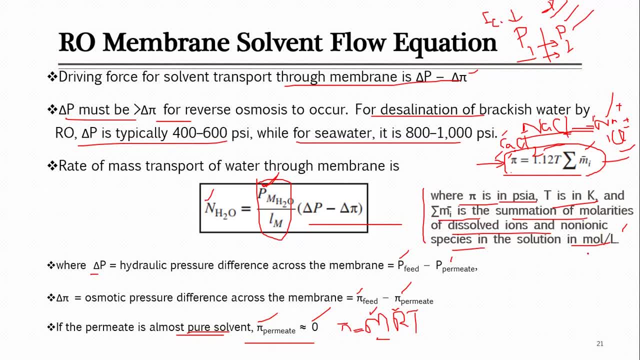 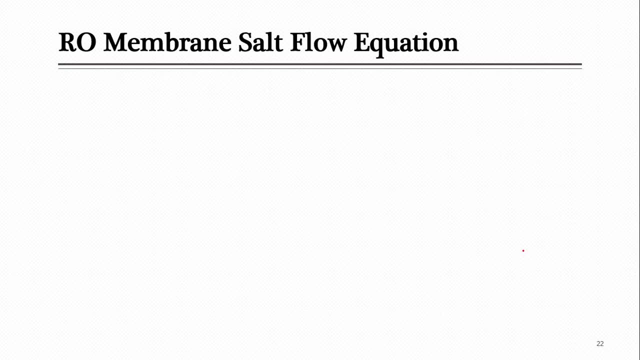 you are using this equation and you calculate molarity yourself, So just convert it to mol per liter. I think we will also make such conversion when we are going to use this equation today, but take care of the unit, like pi, Should be in psi, t in kelvin and this in mol per liter. So this was equation for solvent. 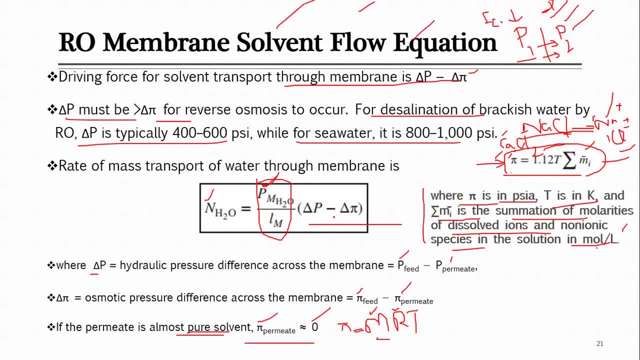 flow calculation and I have explained to you the various terms inside this. So most of the time pressure this may be, you will be thinking how to calculate this pressure across the membrane is most of the time provided, or you can. you can see that we can actually. 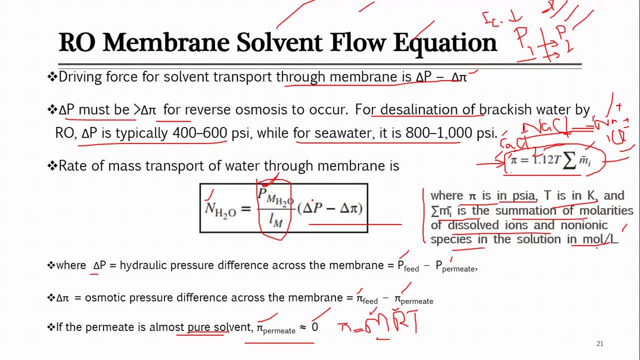 measure this pressure across the membrane by just inserting like pressure gauge. But this osmotic pressure that is due to salt, You have seen, and due to based on temperature. So you can see this salt are accommodated here in molarity and temperature is available in its relationship. So that is calculated. 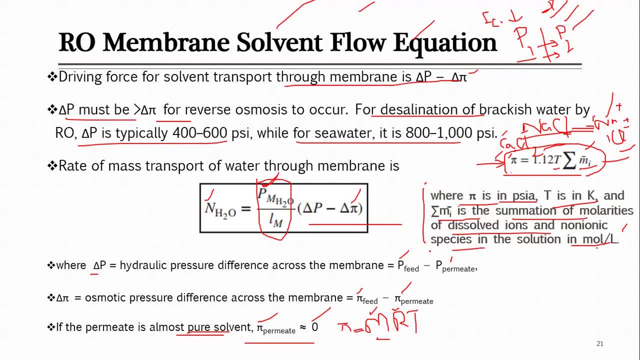 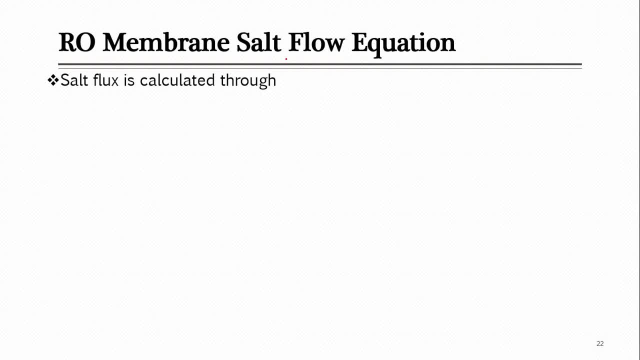 by using equation and most of the time when you are designing the system you have to calculate. Other is salt. we saw that another second parameter, that salt calculation and salt flux is calculated through some equations. They were already described in some section which we have skipped. 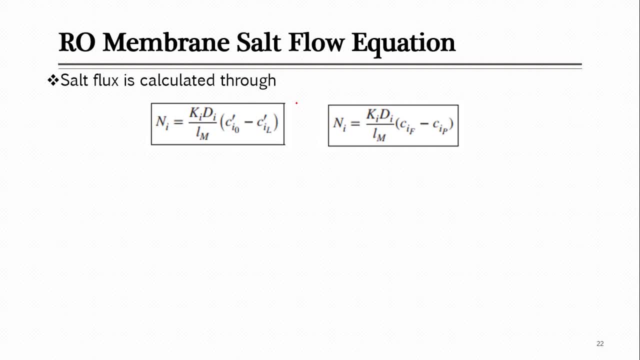 a little bit, which is about salt transfer. that, as I told you that that was not, I mean, related to you or your course, But one equation which can be used for salt flow calculation in this section, even for RO. So that is this equation, same equation. So I will just explain. 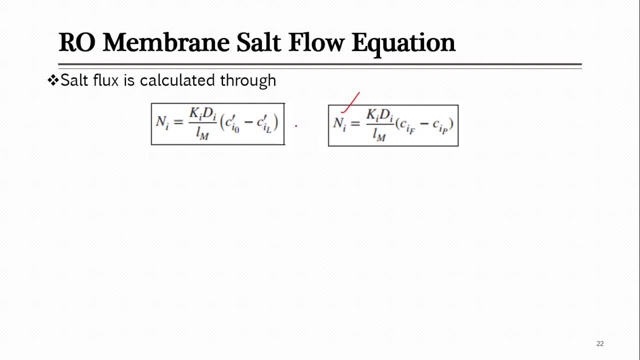 this because they they are, they are similar. there are just few. I mean based on given concentration. this equation can be modified like here, that is, C I naught and C I l, But but the only one equation which can be used here is what is known as the HAL. 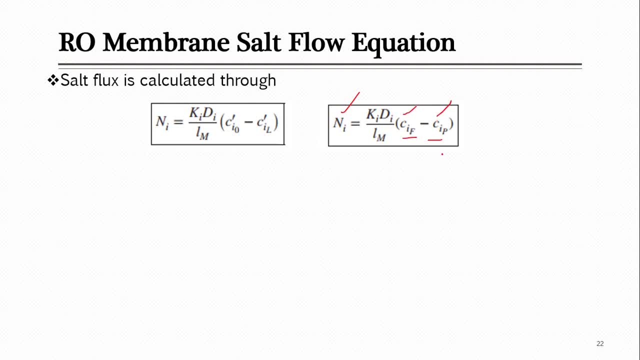 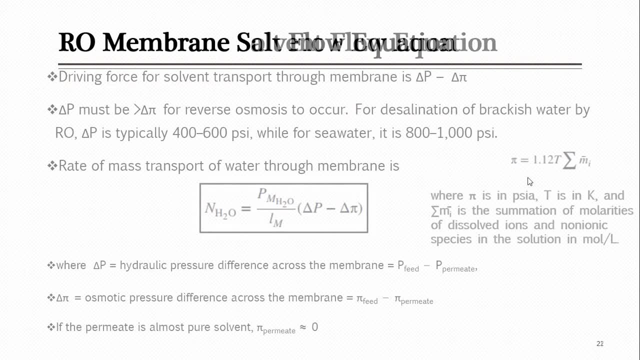 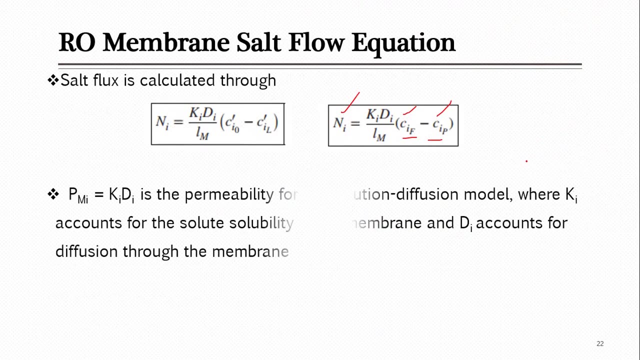 usually we have feed and permeate and their concentration We also calculate, because concentration, actually molarity, is also a unit of concentration. So when you will be calculating here the molarity for solvent flow rate, definitely you have calculated this molarity and that can be used again in this equation. due to this, I will adopt this part of the equation. 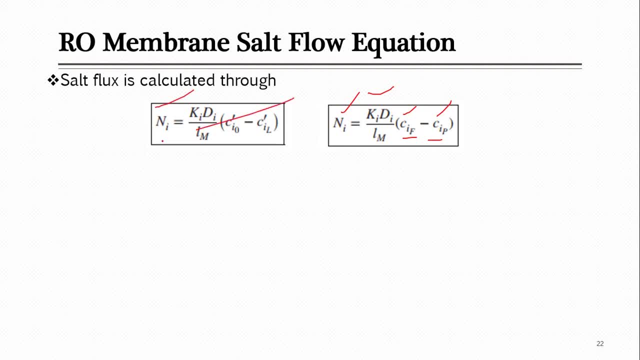 I will not use this equation So you can just skip this equation. just look at this equation here overall. you can see again, for any salt, any salt component, if you are calculating its flow or number of mole through some membrane, So that will be equal to this is again here. 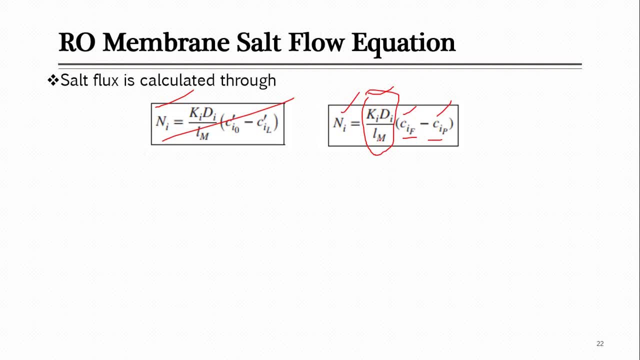 the permeance, that is, permeability divided by thickness of the membrane. Here permeability is actually given in terms of mass transfer coefficient and diffusivity. So as I mean other are here, concentration on the feed side of the said that component, as well as the 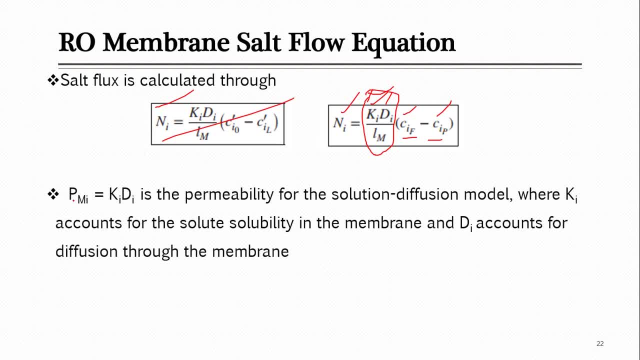 cell on permeate side. So for here, like pmi, this permeance is- you are not sorry- permeance. this is permeability. I mean term which is in numerator, that is permeability, and permeability over thickness is actually permeance. So we are talking about this numerator, that Ki. 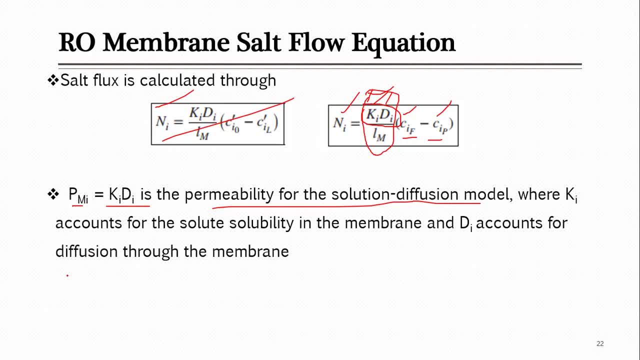 Di is a permeability of solution diffusion model, where Ki accounts for solute solubility in the membrane, So and Di diffusion through the membrane. So if we know these values then we can definitely calculate this permeability and then permeability that that will be used. So these are also measured based on the experimentation diffusivity. 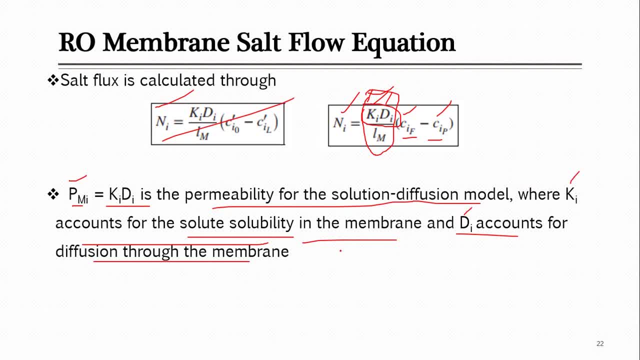 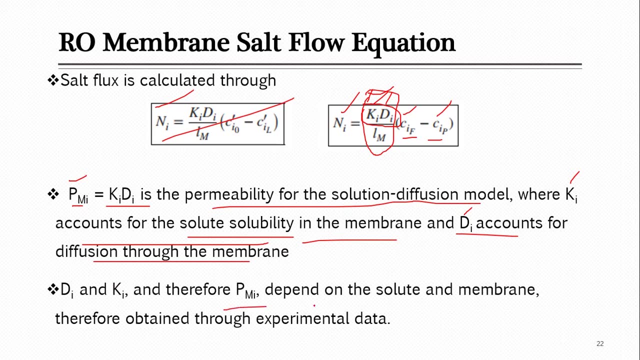 and solubility of various component through the membrane, So all membrane system. usually when they are developed they are tested on the lab scale and all this data is collected. then that is used for designing the system on large scale. So pmi and Ki, and therefore pmi, they depend on the solute and membrane, as I am telling. 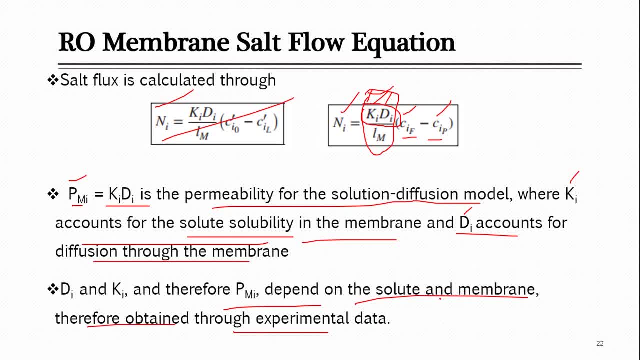 you. they are not specific, they are not like, only general formula for them. So you have to look at the interaction, diffusion, solubility of various component through the membrane and when you will change the membrane material, you will change the solute, they will. these: 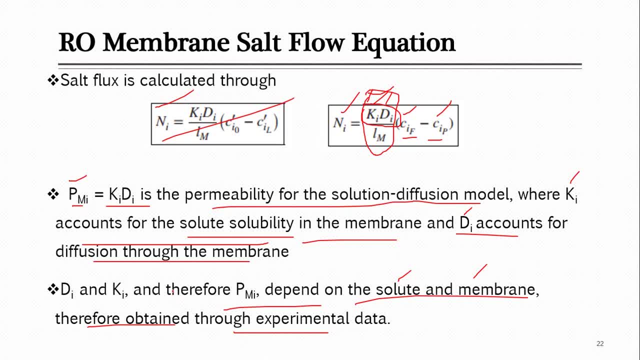 will change actually, So that can be obtained from that data and then they they will be used for making these calculations Otherwise sometime- I mean you are directly given the permeance based on that is also definitely based on the experimental data for any membrane. 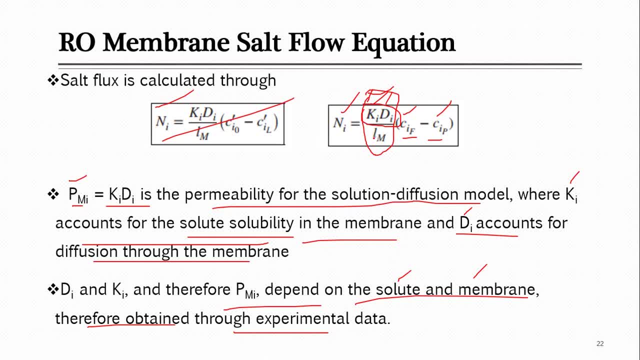 So it is not necessary that in some problem you are not given like thickness, you are not given Ki and Di. that is, direct permeance is given. So that is fine. that is really mean easy for you to use directly permeance here and multiply it with the difference of concentration. 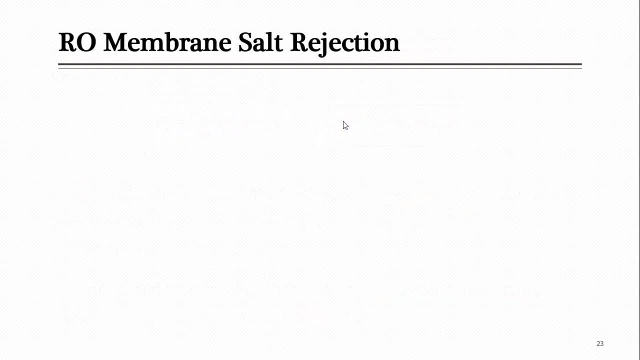 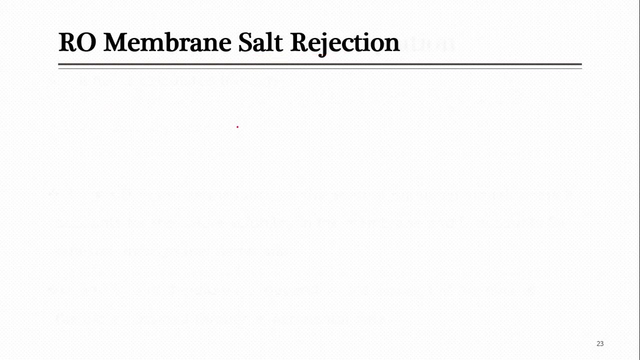 and you can get salt flow rate. There was one term, salt rejection, which we said is important. salt rejection, what does this mean? actually, before we go for salt rejection, we look at the salt passage. I mean here, as in the last slide we saw, that we are calculating the flux of salts through the membrane as 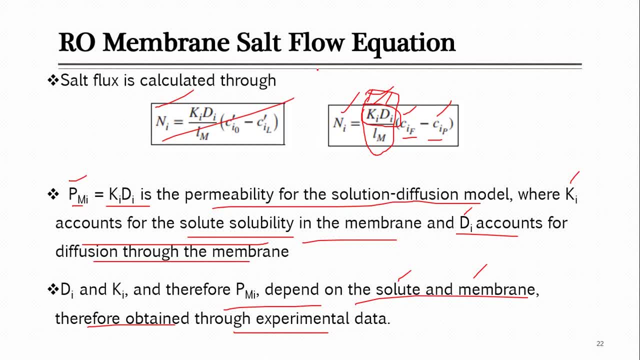 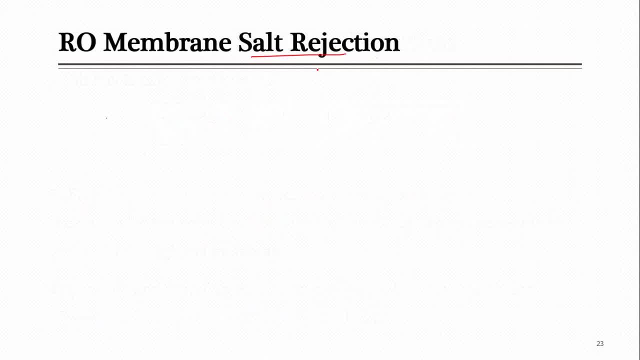 I explained to you that membrane are not 100 percent selective for solvent only. they can also allow some of the other component to pass through, and here salts, which are solute, that can also pass through the membrane, and their flux can be calculated by using this equation. 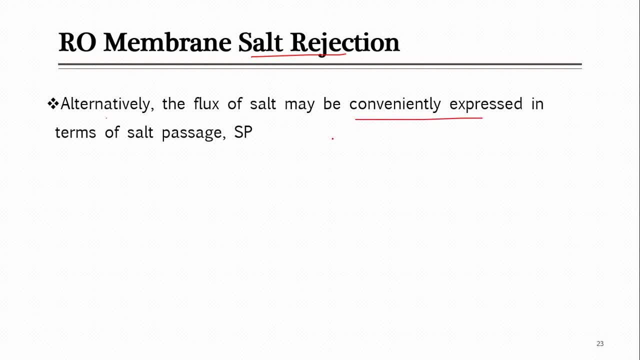 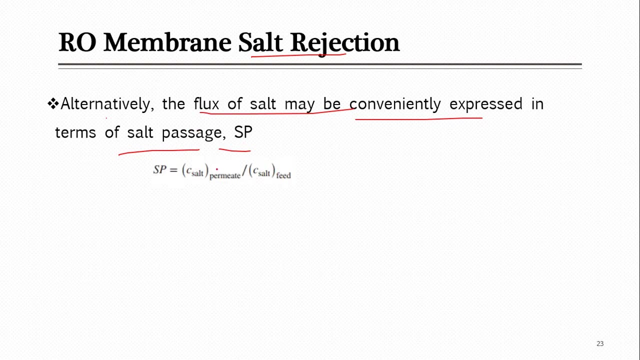 Well, passage of the salt can be also expressed in terms of our flux of the salt. that can be expressed in term of another mean term that is called salt passage, SP. this represented with SP in your book- salt passage, and that salt passage can be easily calculated if we 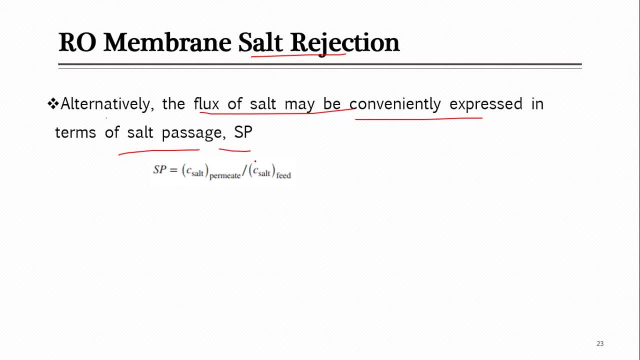 are just looking, for example, the fraction of salt which has passed through the membrane. So that is like concentration of salt on permeate side over concentration of salt on feed side. So we know that if we know or we have these two values, all passage can be easily found. 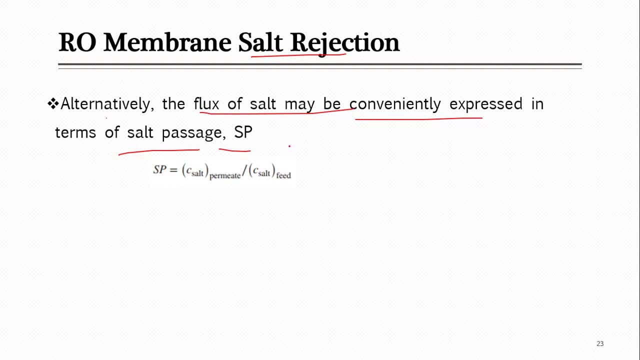 that how much percentage. if we just multiply it with 100 we can calculate percentage. otherwise it is fraction can be found. And when you know that, suppose if you know the amount of salt on feed side, suppose we just consider it that is 1 or 100 percent, So sum of that portion has passed through. 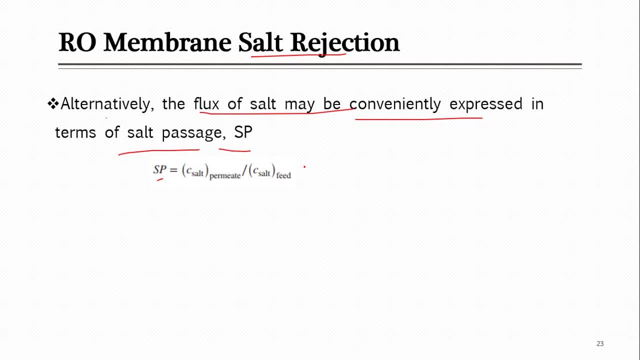 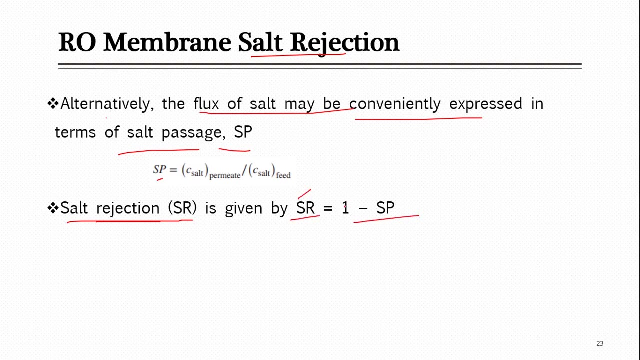 this membrane. for example, 5 percent has passed Overall. how much is rejected are not allowed to pass through the membrane? that's called salt rejection mean all those salt which was rejected which were not allowed to pass through the membrane. so that is represented with. sr is equal to 1 minus sp and 100 percent like sp. 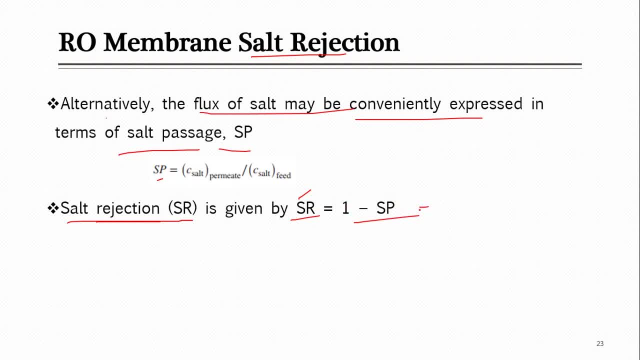 how, which was possible? 100 minus 5, it will be 95 percent salt are rejected. so most of the time membrane which you are using- they they like- don't allow much salt to pass through they. sometime you can find 2 to 3 to 5 percent salt can pass through the membrane. all other are rejected. mean and 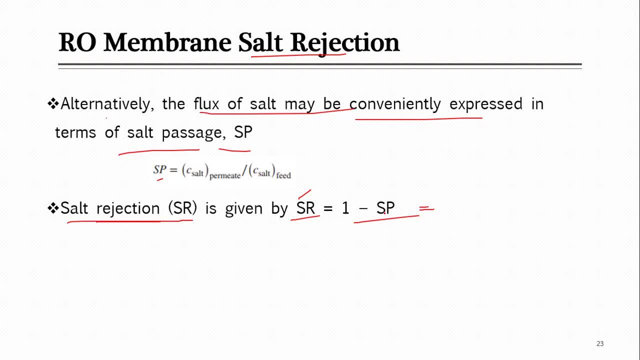 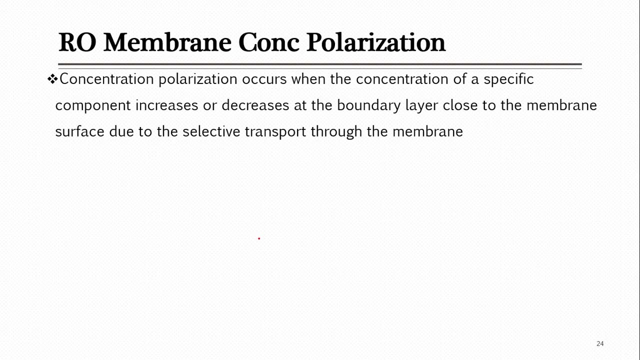 definitely the membrane which will have more salt rejection will be more good membrane, because we want to separate solvent from the salt and if they can't pass through the membrane, definitely that membrane system is good right. next topic is related to concentration polarization. so what is concentration polarization or important factor across this? this also appeared in. 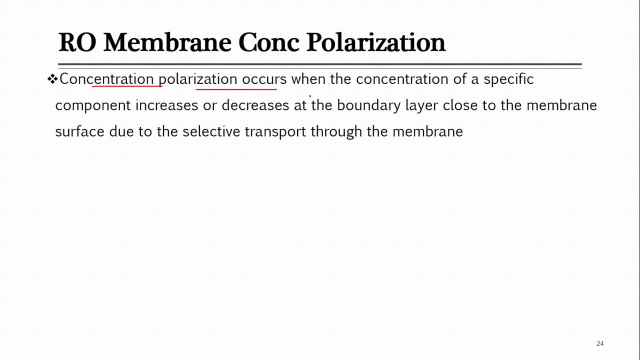 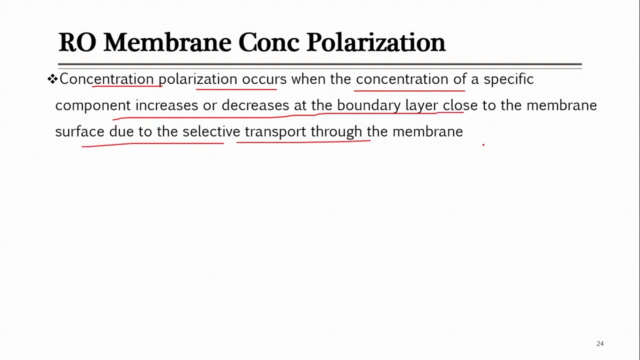 the lecture about membranes i think in in this week. so concentration polarization: as its name indicate, polarization, creation of some pole, something like charge. so concentration polarization occurs when the concentration of specific component increases or decreases at the boundary layer close to the membrane due to selective transport through the membrane. 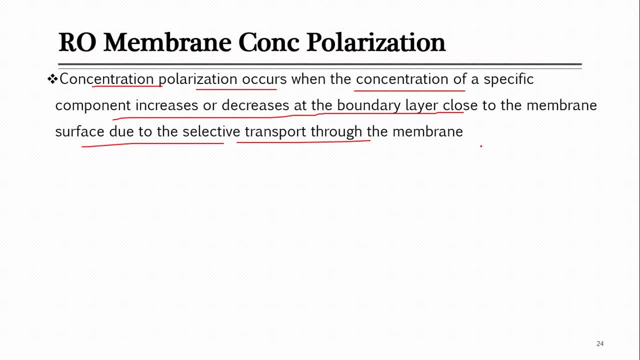 as we know that we only allow or we are looking for solvent to pass through the membrane. so all salts will be rejected at the surface of membrane. so they start building. and when they are building at the surface, definitely they, if they are not removed through the system. so their concentration is increased and this phenomenon cause actually concentration. 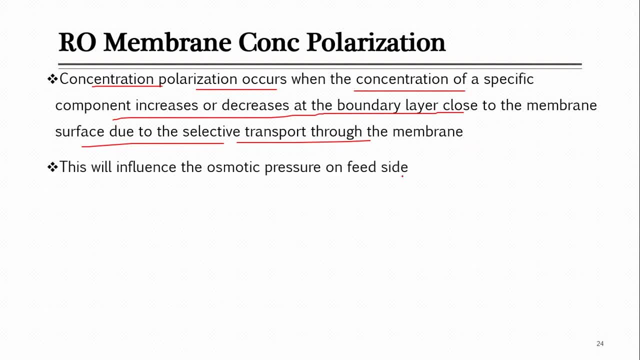 polarization. and it is important why? because we have seen that osmotic pressure across the membrane that's highly dependent on the salt concentration. if salt concentration is increasing inside the system, so that will increase the osmotic pressure and membrane performance will decrease. so due to this, 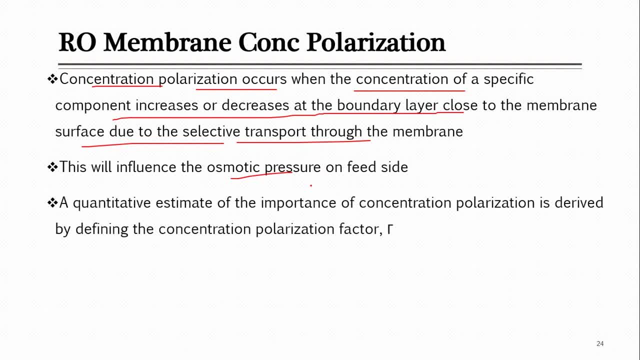 it is important to calculate or look at this concentration polarization and that concentration polarization can be calculated, or i mean there is a again derivation for this quick derivation, but we will look at the final expression that can be used for calculation of concentration polarization factor. so that's represented with this symbol. so 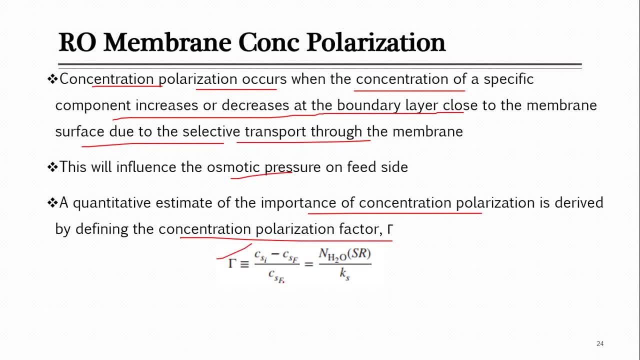 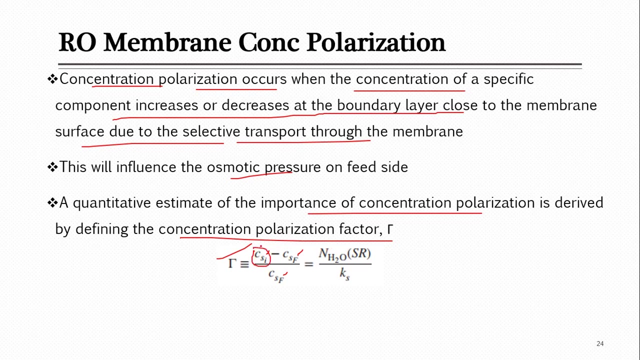 that's something concentration, polarization is equal to like. these are again concentration of any component, mean at interface something, feed- and again mean concentration of those salts inside feed as well as at the interface or boundary layer. so this is again difficult to find or calculate. one thing here, actually: 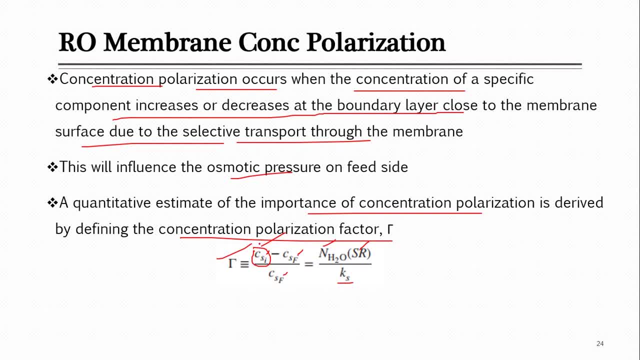 this concentration, CSI, as it is difficult to measure. So that is another replacement formula here. that is about flux of solvent through the membrane, which you have already calculated. salt rejection: that is also calculated by using salt passage and then Ks, that is this salt mass. 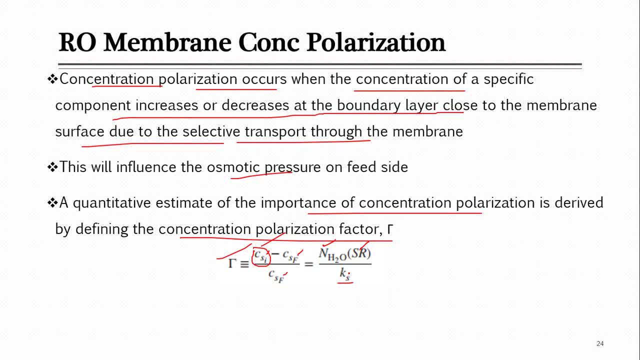 transfer through the membrane. So this formula can be used to calculate this concentration polarization. So when you are designing any reverse osmosis system, it is important to calculate this parameter for your given system based on your requirements. So value of usually 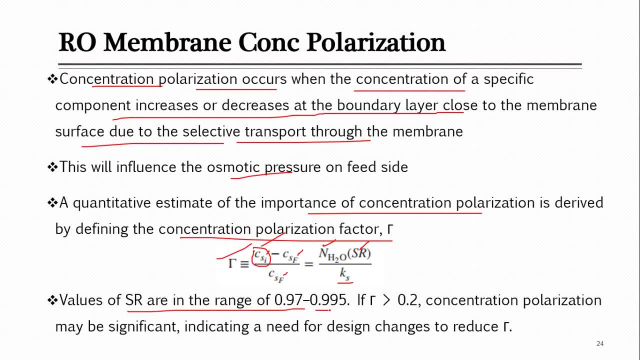 salt rejection are between 0.97 to 0.995.. This means, like salt which only pass through the membrane, range from 3 percent to 0.5 percent. otherwise, 97 percent to 99.5 percent salt are rejected And if concentration polarization 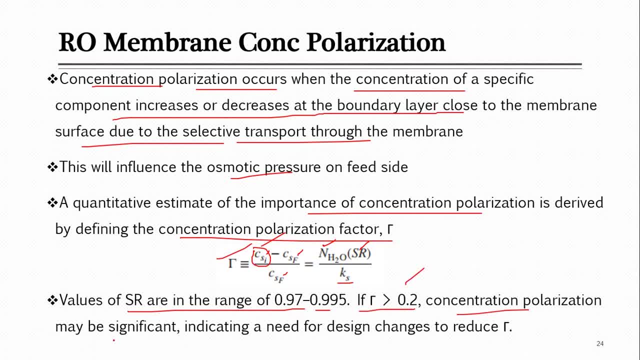 value is greater than 0.2, then concentration polarization is significant and it will create high osmotic pressure. due to this, you will need to design the system or change the system in which will reduce concentration polarization. So when you make calculation and its value is, 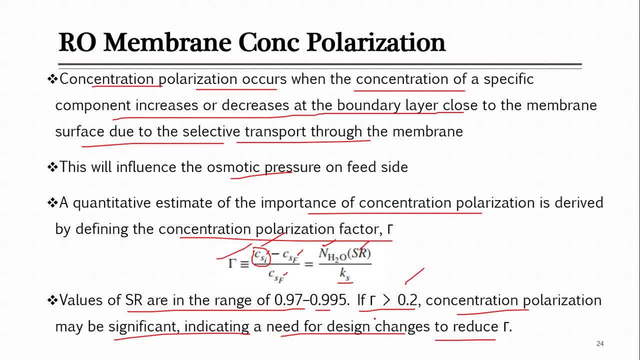 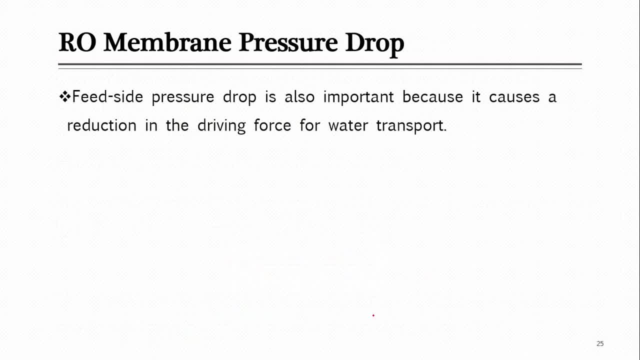 greater than 0.2.. So it is important to may remove those salt, to reduce the concentration, polarization or change the design of your system. The last parameter which is important, that is about pressure drop and in pressure drop, actually this feed side, pressure drop is important. 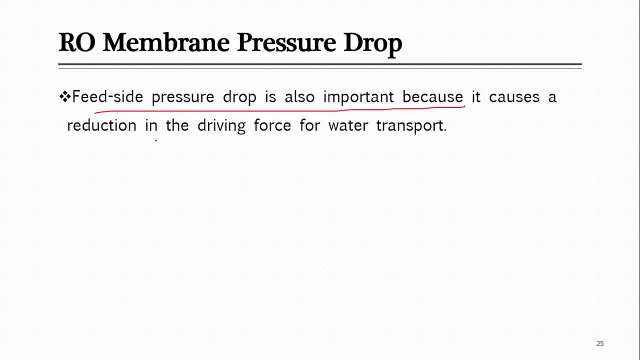 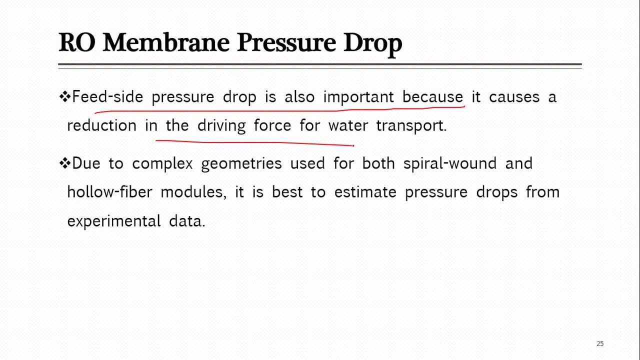 because we have seen that that is the major cause of driving force through this membrane. So if pressure drop is higher through the membrane, So then there will be problem. the problem, actually, it will not provide you sufficient permeate or the separation which you are looking. 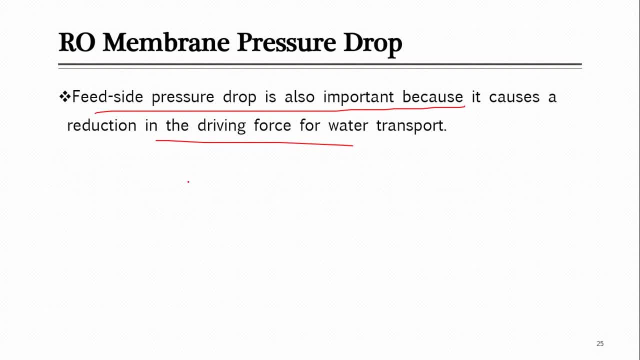 for. But as we have seen here- I mean sometime- you have seen that pressure drop can be calculated for various equipments Through even columns, through, like as we have seen, plate tower, through packed column, but through this membrane system, especially RO membrane system, it is difficult because there 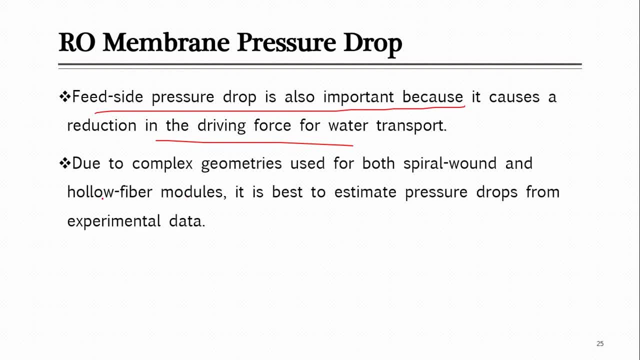 are difficult geometries of spiral, wound and hollow fiber membrane So the equations are difficult to manage and they cannot predict good pressure drop calculation through this RO system. So it is better to estimate the pressure drop. So it is better to estimate the pressure drop. 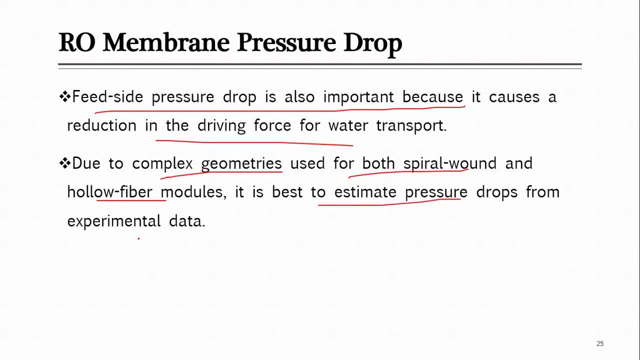 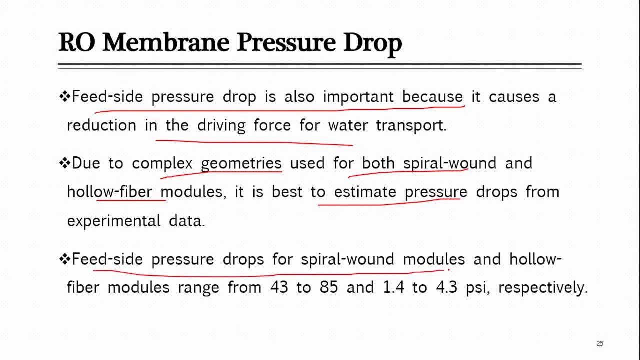 plants. So feed side pressure drop for spiral wound module and hollow fiber module range. there is some range like it should be like. if you are using spiral wound you know that spiral wound modules there are the sheets which are rolled and then there is one tube at the center. 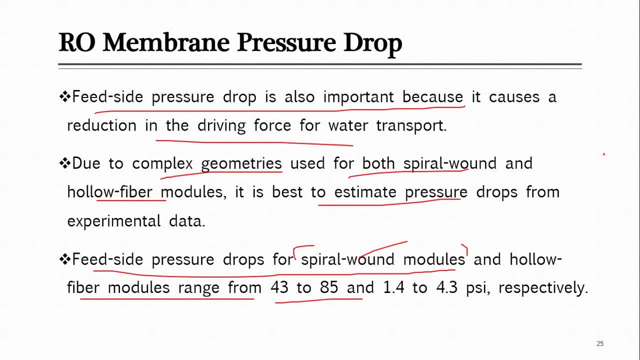 of these I mean rolled, I mean rolled membrane. so that's a complex system and in that pressure drop is high. it is allowed, like pressure drop, from 43 to 85 psi, while in hollow fiber module that's less. actually they are hollow fiber, very small fiber. there are very small holes through those fiber and 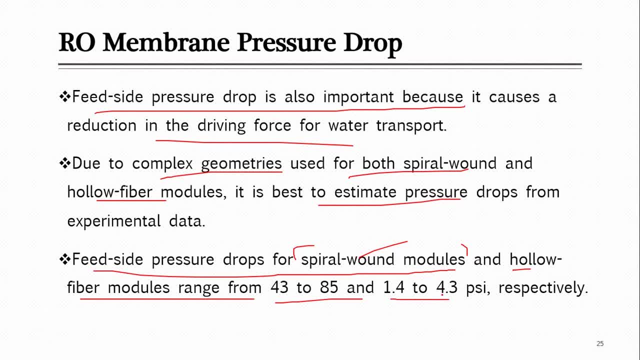 mean this separation takes place and there it is only 1.4 to 4.3 psi. so just overall, you can remember quickly to this like it's around 40 to 80 psi and it's 1 to 4 psi. so that's not calculated. 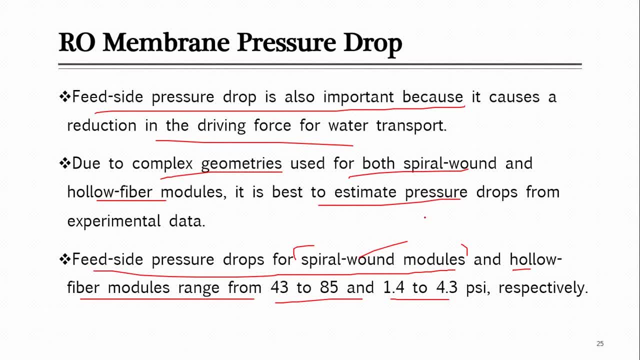 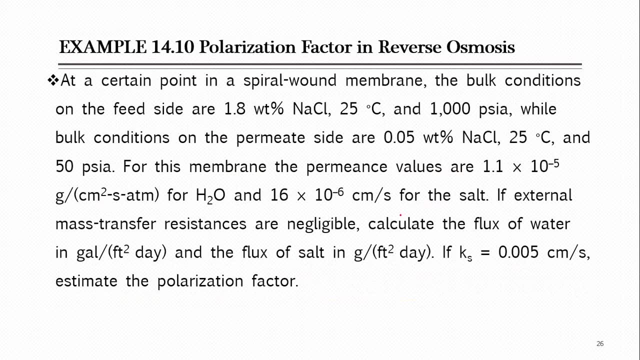 due to this, when we are going to start this problem, in which we will not calculate this pressure drop but all other, we will look at those parameters that they we have to calculate. so here i am going to discuss this example quickly. so i have tried to make it simplified as compared to the solution provided in the book. so 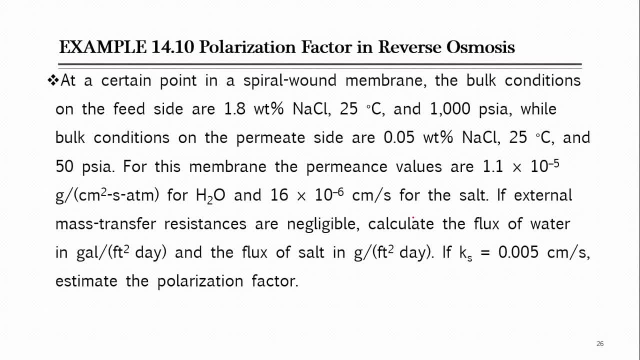 let's proceed with this. actually in this example. by the way, up to here we have discussed major, important parameter which are considered during design of the membrane, RO membrane system. so they include solvent flow rate. you have to calculate permeate solvent which passes through the membrane, for example, water flow rate as well as salt flow rate through the membrane. 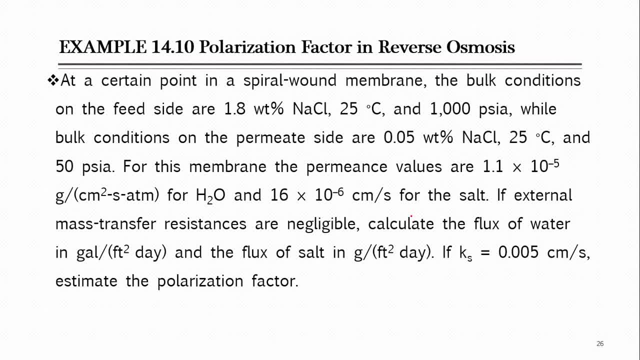 through the membrane and then we have to calculate the permeate solvent which passes through the membrane, then salt passage or salt rejection calculation, and actually we are calculating it to calculate, finally, concentration polarization across the membrane. so let us look at this example here that i mean, that's about calculation of 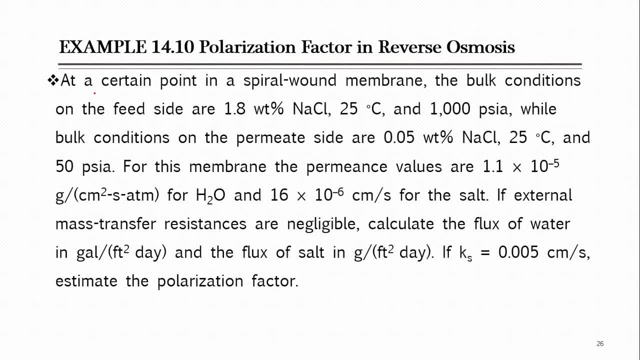 polarization factor in reverse osmosis at a certain point. i mean, there is spiral wound membrane and you know that when we are using these membrane there are various modules and number of modules. but here he has provided for, like suppose, there are many spiral wound modules. they are being used as a RO filtration plant or RO membrane plant. so in that you have, you are. 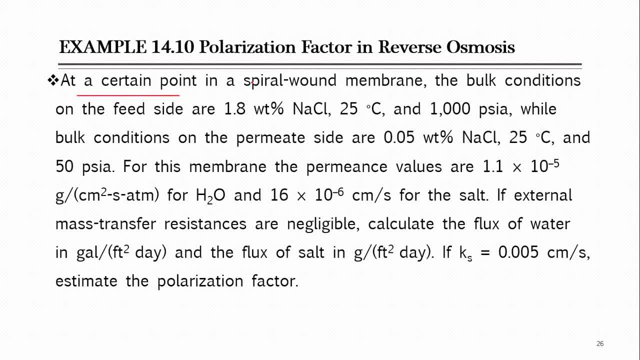 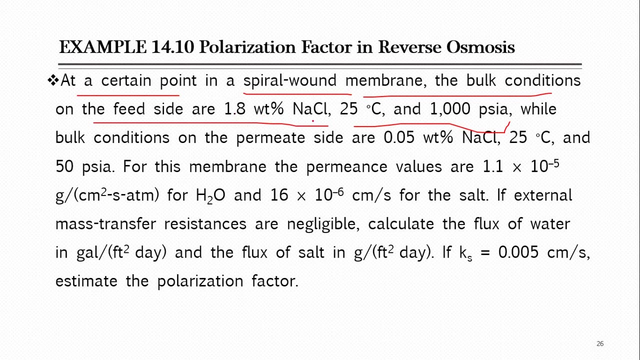 making calculation at certain point. at a certain point in spiral wound membrane the bulk conditions of feed side are mean if you look at that system, in that system, feed side conditions, feed side condition mean, feed water, temperature, pressure and composition of the feed. so that feed contain 1.8 weight percent NaCl. so, as I said, I, as I told you that most of the time reverse osmosis membrane. 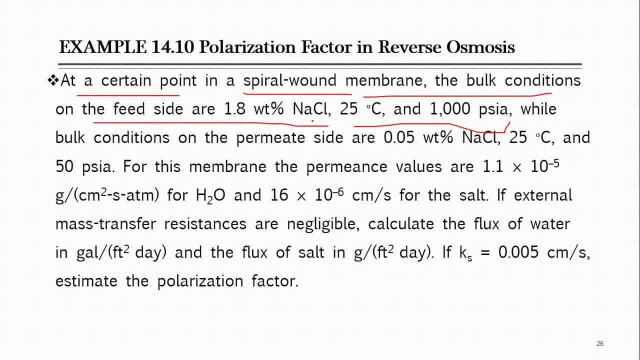 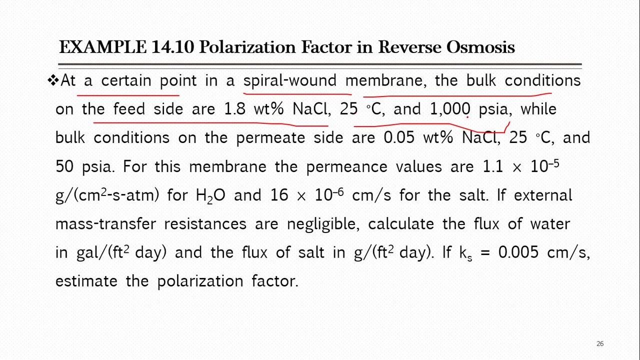 are used for desalination. so here he has provided as a clear example of desalination, and in this you can see that he has only provided you the only NaCl concentration rest. he did not talk about anything else. so let us see that. So later in this problem he will talk about water, but like here, 98.2 percent will be water, 1.8 percent is NaCl and 98.2 percent will be weight percent. based on weight percent that will be water, and this is available at 25 degree C and 1000 psi. 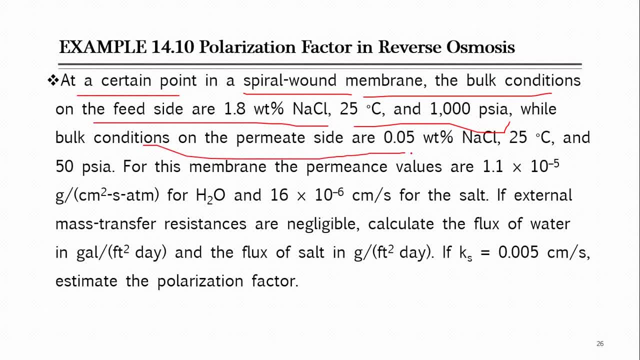 While bulk condition on permeate side are 0.0 weight percent NaCl, it is mean only- I mean this- 0.05 percent NaCl. If NaCl passes through this membrane, it is mean 99.5 percent water will be there at. it is available at 25 degree C. mean temperature is same on both sides of membrane but pressure has highly reduced. it is only 50 psi on the other side of this. it is only 50 psi. 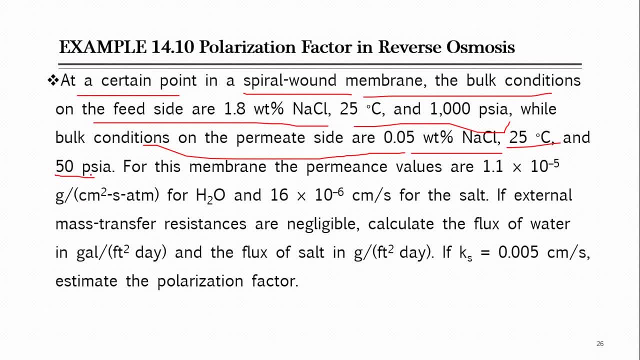 Then there is for this membrane. the permeance values are here. they are also given like directly permeance value for water. Like directly permeance value for water, That is 1.1 into compress minus 5. that was actually permeability divided by thickness of membranes. 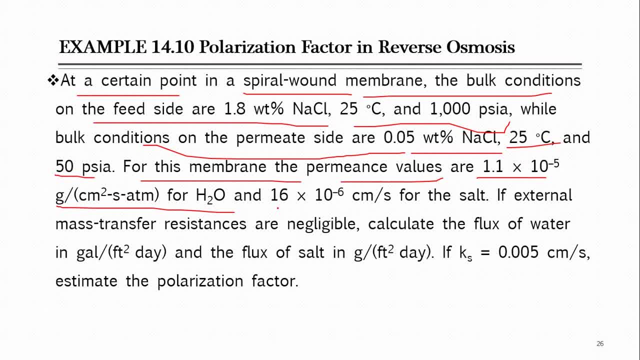 So that has directly given to you as a some things of the water and also 16 into 10 to the minus 6 centimeter per second, for the salt means all NaCl permeate fall. That is also given. so that is good. Like directly you are given with the permeates. you do not need to go for permeability and thickness and all of those calculation have. 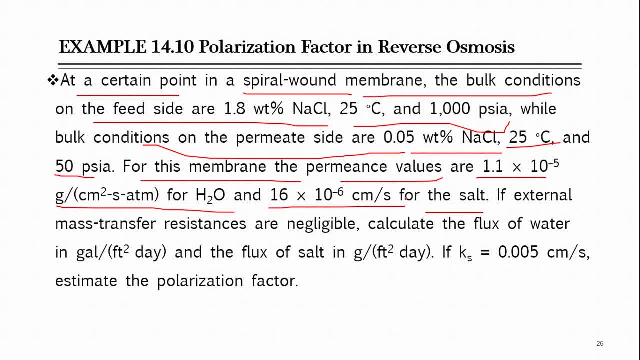 People does not have to do For that very can be caltion or 10 to the minus of 5 meter per second For a calculation of k and d and all other stuff. If external mass transfer resistance are negligible here, no mass transfer resistance is mean external across the system. So calculate the flux. 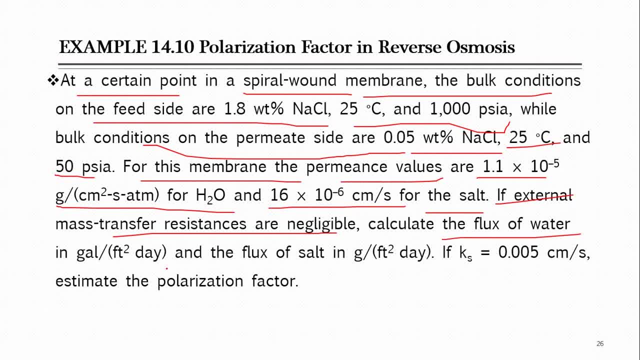 of water. we have to calculate flux of water and he has mentioned the unit in gallon per feet square per day. and then there is flux of salt. I mean, you know, flux is flow rate of something per unit area of the membrane, So it is gallon per day, I mean flow rate. 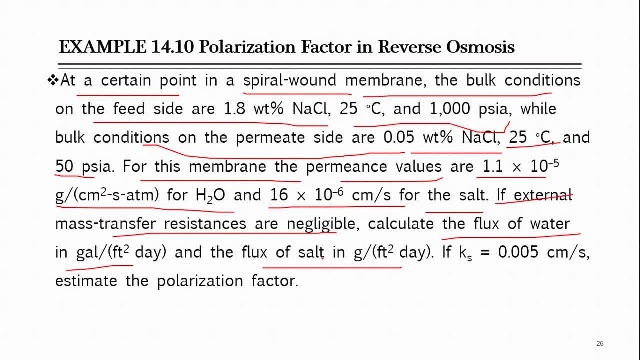 of water per feet square of the membrane. and then salt. you know salt is measured in gram, that solid stuff, So that is in gram per day per feet square. that salt flux we have to calculate in gram per feet square per day. If k s, that was 0.005 centimeter per second. 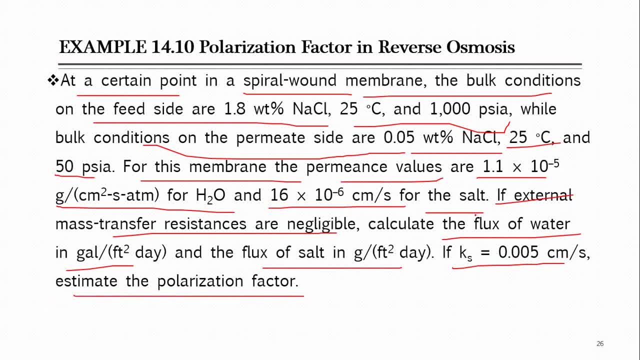 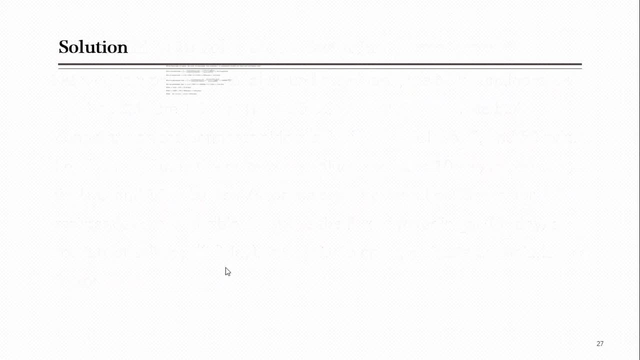 estimate the polarization factor. So, overall, you can look at this based on this given data. finally, we have to calculate three parameter, that is, flux of the water, flux of the salt and concentration polarization. these we have to calculate. So let us start with the solution of this problem. first of, 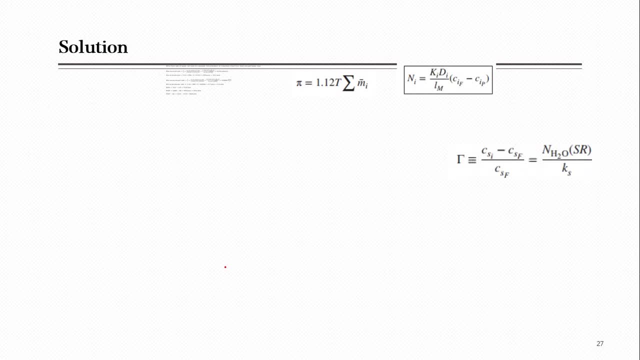 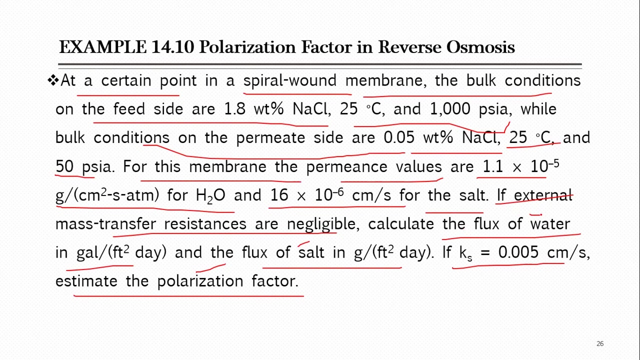 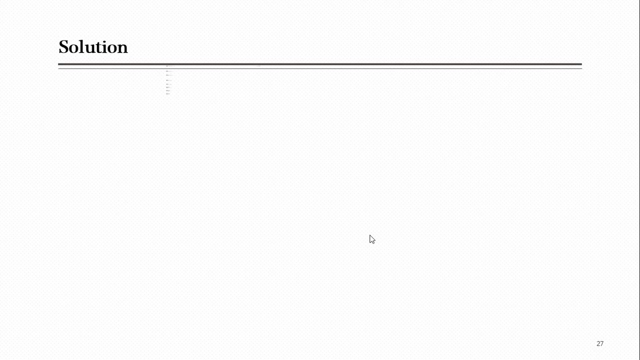 all, Let me tell you here you have to use three different formulas. So the first one is where the driving force of delta p minus delta pi- So out of this permeance- is already given to you. then there is delta p pressure on the both sides of membrane. 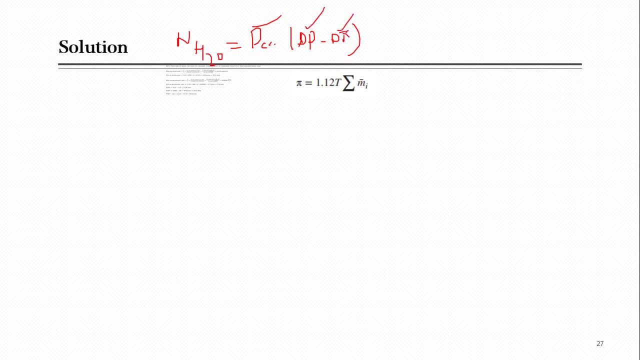 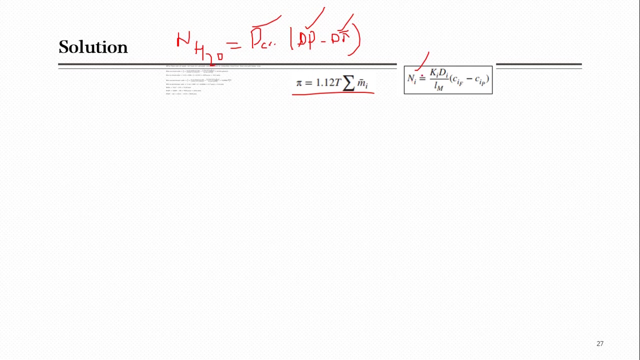 is given, So this can be easily found. then there is delta pi, that is, osmotic pressure, and due to this I have provided you the equation which we have already talked. this will be used for this calculation, And then this formula will be used for calculation of salt. I mean flow rate, salt passage salt. 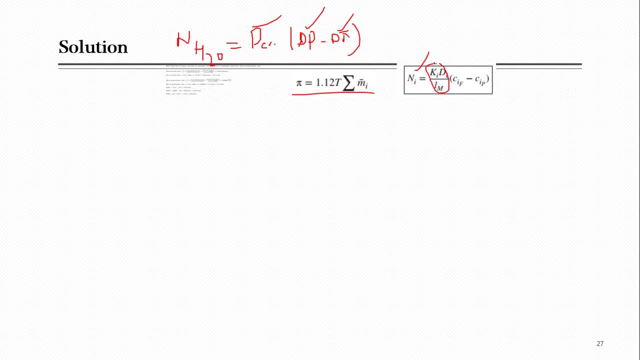 flux through this membrane. And then we have to take the solution of delta p, So which? So that is permeance, this parameter, as I told, this is permeance, So that is already given. So what we will need, we will need concentration of feed and permeate side to 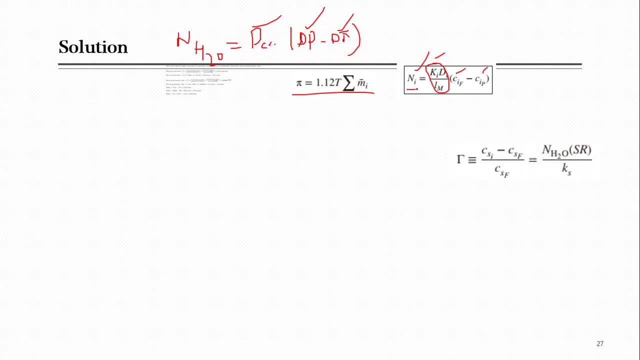 calculate this salt flux through this membrane And then finally, you have to calculate this concentration, polarization, So you can use this formula, this side, So that is mean flux of water. when we have calculated in the first part, that can be used here and then there. 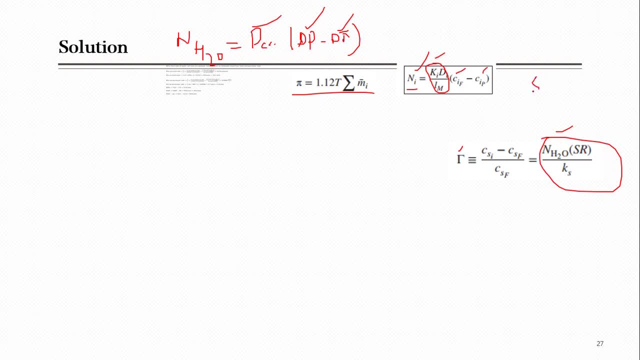 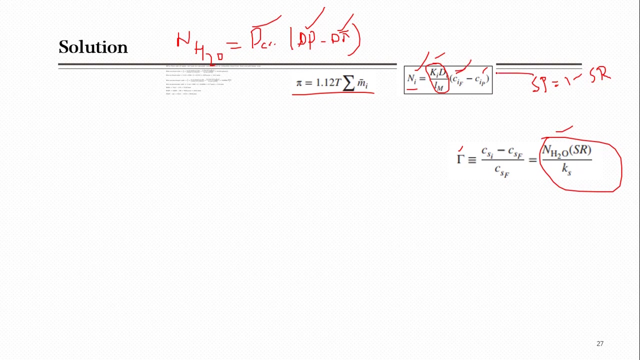 is salt rejection. So salt rejection will be calculated by using: sp is equal to 1 minus sr and sp can be easily calculated because you know that sp was just the ratio of concentration on permeate side over concentration on feed side. that can be easily found, as we have already. 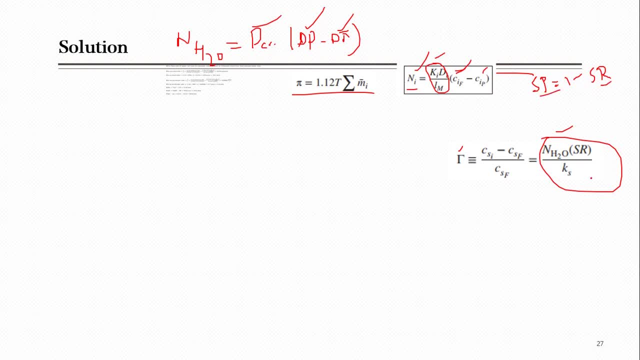 calculated this stuff. So sp will be calculated with this sr and this ks is given. So these are 3 or 4 formulas which you have to use for these calculations. So that is all, Thank you. So initially, let us start with the calculation of water flux. For water flux, if you look. 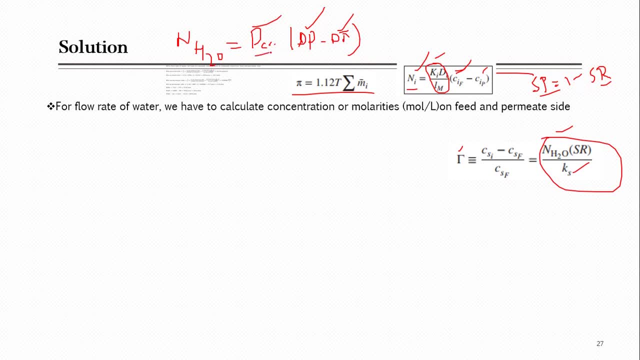 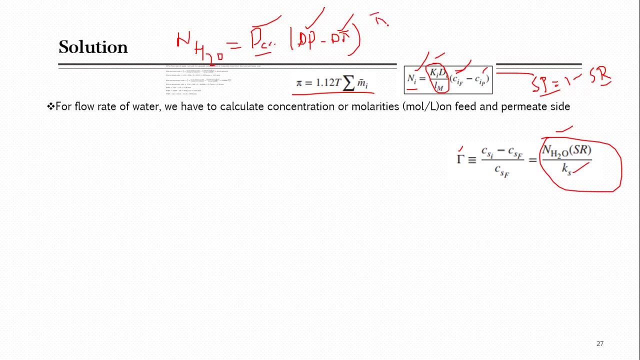 at this formula, as I told you that in this permeance is given, delta p is given to you, then the only thing which you need to calculate, or you should know, that is delta pi. And for delta pi it is mean that is pi on the feed side minus pi on the permeate side. So you 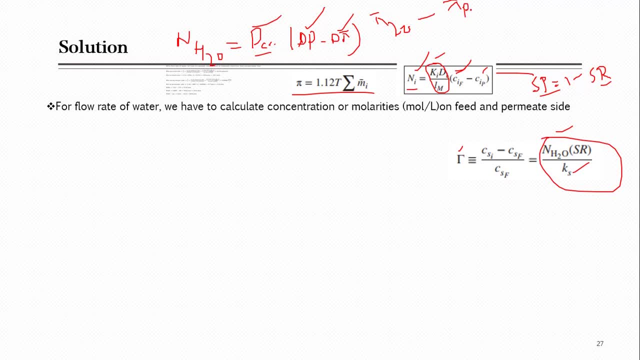 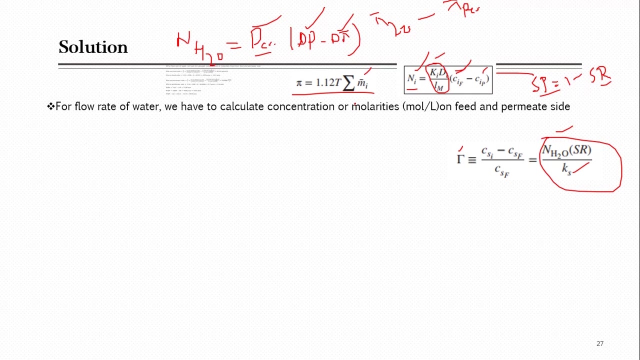 will need pi on both side, permeate and feed side- And in order to calculate this formula, this pi, you know that here, as per this formula, you will need to calculate molarity on both side, mean, feed side as well as permeate side. So let us mean look at this for flow rate. 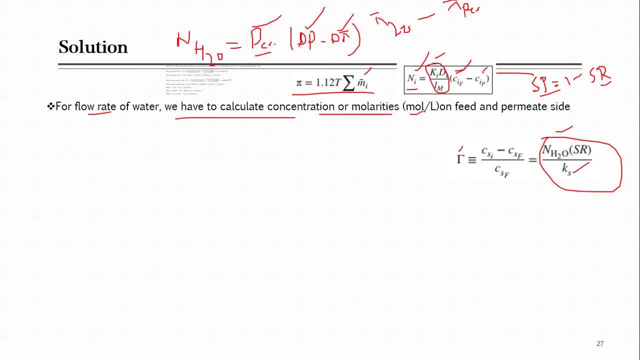 of the water, we have to calculate concentration of molarity and that is unit, is mol per liter for feed side and permeate side, which I have just explained to you For this calculation. so how we can calculate molarity on the feed side that is equal to: 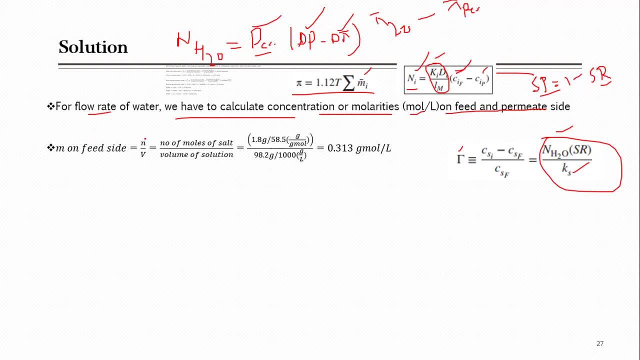 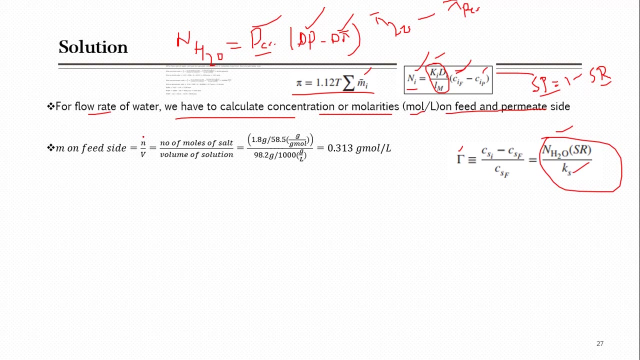 actually number of moles over number of moles of salt actually over volume of solution. this is the formula for molarity. just remember, Currently I am explaining this in the book. it is not too much clear. So I mean, just look at each and every step carefully so that 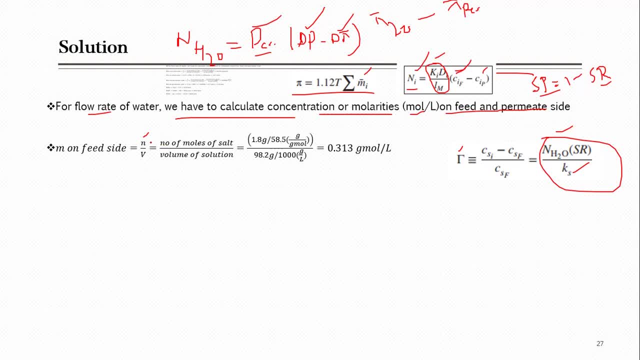 you can later solve other problems. So number of moles: how we can calculate number of moles of salt? do we have any amount of salts here? Yes, if you go back to the question that we have seen in the previous question, So based on given data, there was 1.8 weight percent. 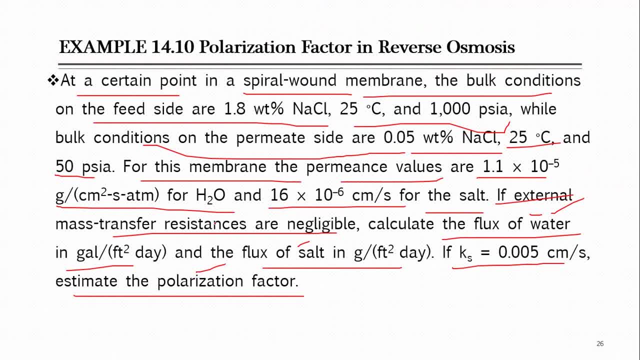 NaCl. if we take it like 100 percent feed side, I mean mass flow or percentage 100 percent, So it will be like 1.8 percent, or if I consider it as a like 100 gram on feed side, So out. 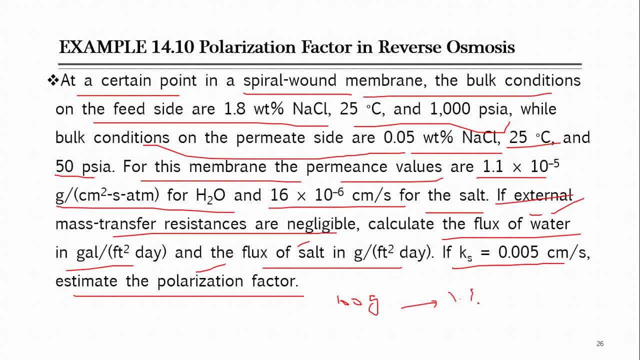 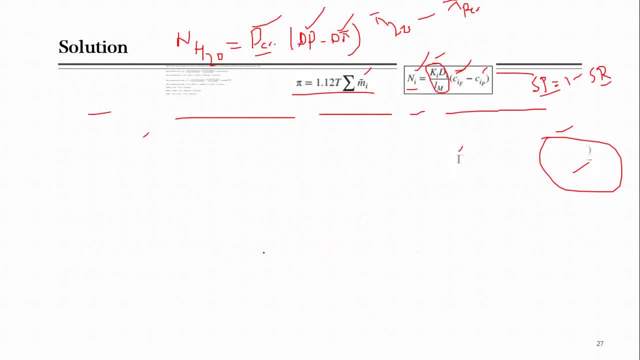 of 100 gram, NaCl is 1.8 gram and other, like 98.2, is water. So this is the total weight of the water. So let us use this, I mean 1.8. this number of mole, you know number of mole is equal to. 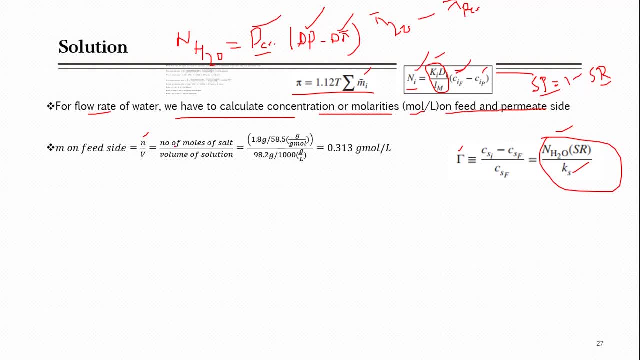 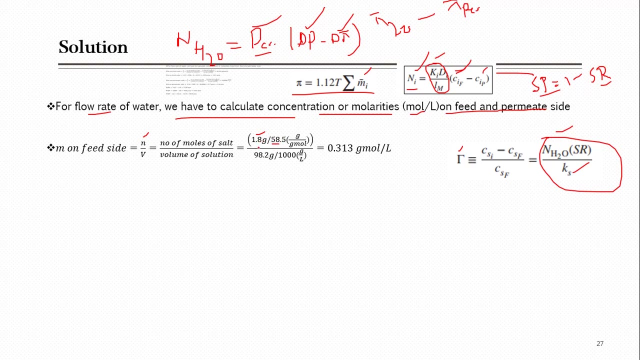 mass over molecular weight and for NaCl- you know this, I mean mole, sorry- molecular weight is 58.5 and 1.8 gram NaCl was there. So from here you can calculate that it will be like 1.8 gram divided by 58.5. number of moles of salt are calculated clear. 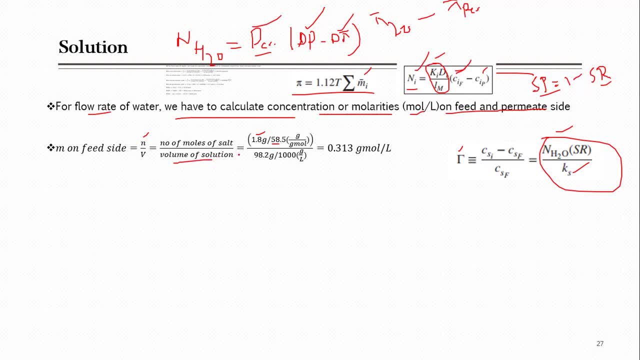 Then there is volume of the solution and solution here is based on the water. So we can calculate volume, can be calculate based on the given data. Yes, somehow you are given some information and that is main amount of water. based on this percentage, that is 98.2 gram. So we can use that if we have the mass of 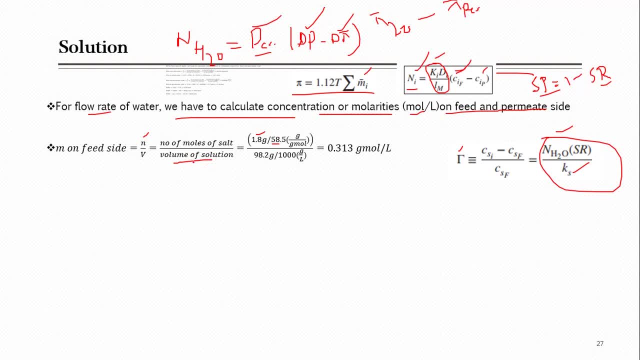 water. we can just divide it by the density of the water and we can calculate volume. by the way, Here some of you will think about it that this is just volume of solution, but using the volume of the solute. Actually, if we just consider even this small amount of, 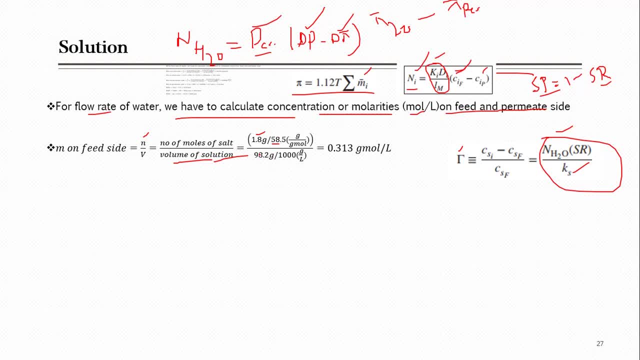 this NaCl, its amount is also accommodated and its density, So that will not make big difference. So due to this, you can directly calculate this volume of the solution based on volume of the solvent that was water. If you have to look for exact, accurate calculation. 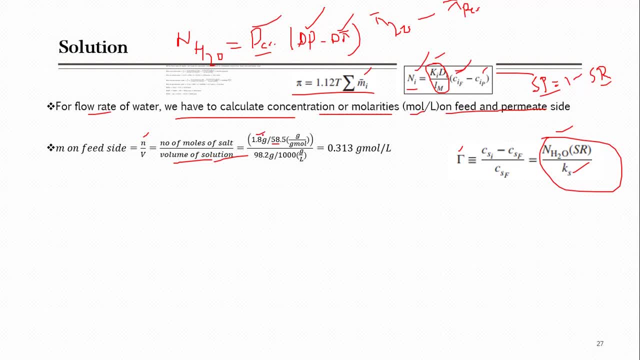 then definitely you will need to include this for volume of the solution, So that will not make big difference. Actually, if you have to even include that, that will not make big difference. So we are directly using only the solvent water. Water is 98.2 gram and 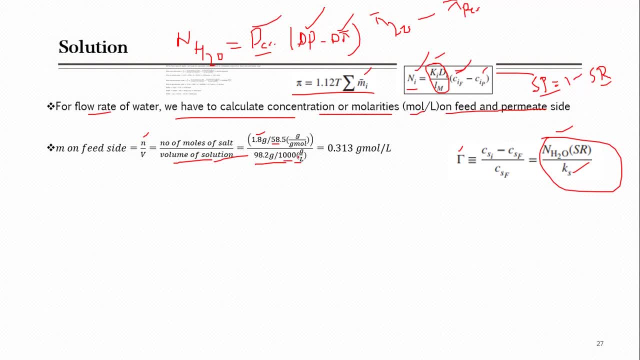 its density in these unit is gram per liter, that is, 1000 gram per liter, And here I mean even you can start with that- 1 gram per cubic centimeter. So you will finally reach to this point. Why? because at the end of the day, this molarity should have unit of mole per liter. 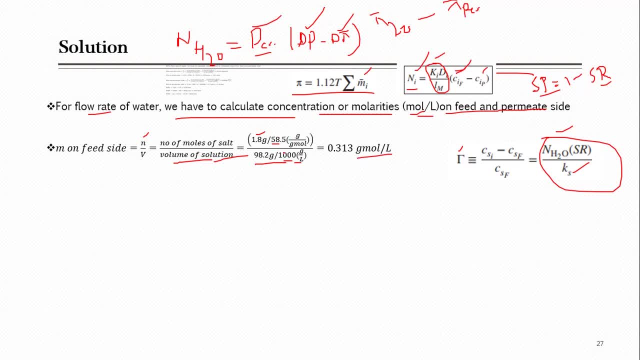 So due to this, I am using, I am using this density value. So overall this gram will cancel with this gram as well. on numerator side, this gram will cancel with this gram And finally, your units which are left are gram per mole and its value is 0.313.. So you can check this calculation Then. finally, 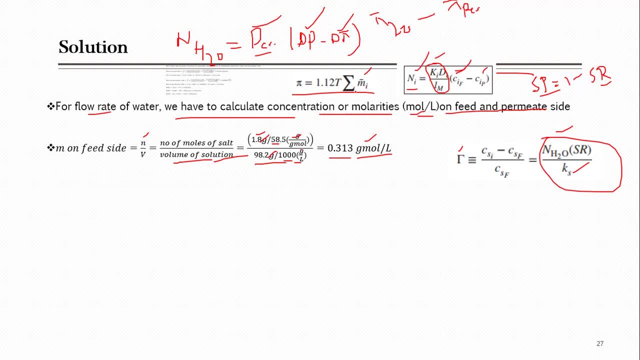 I mean when you have calculated this molarity on feed side. So now that can be used for main calculation of this pi. Because if there is only 1 mole, NaCl, as I told you, if for NaCl 1 mole you are producing, 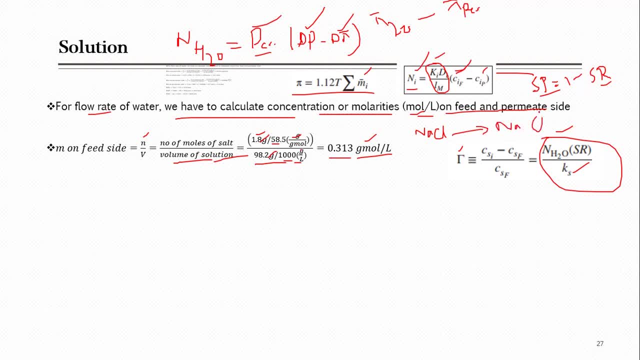 actually Na plus Cl. these are produced. These are this equation. I already told you that that is based on components of salt. So NaCl is giving you Na plus Cl. So here, as we have calculated for molarity of NaCl, So that will give you Na plus Cl, So there will be. 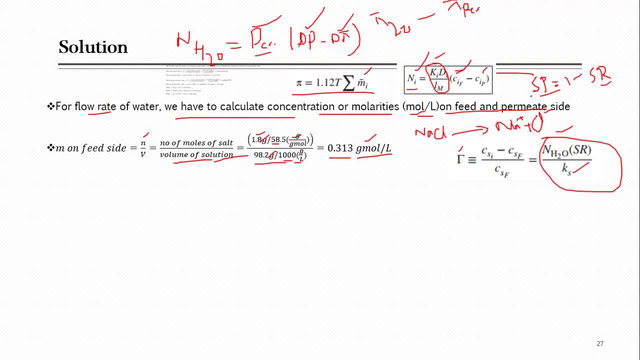 if you have to look for this Na and Cl, So that will be 2 times NaCl, because this 1 is giving 1 Na plus 1 Cl. So based on this, we can use this value of pi to calculate this. pi is equal to 1.12 multiply by temperature. 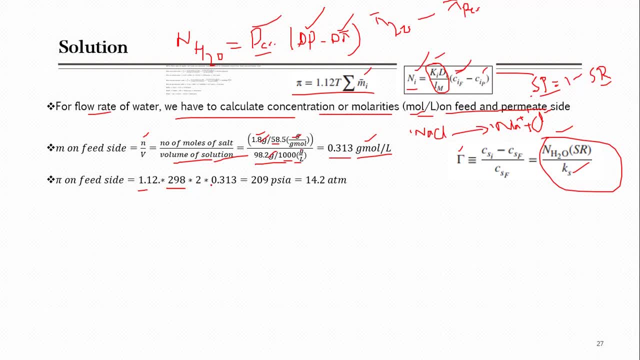 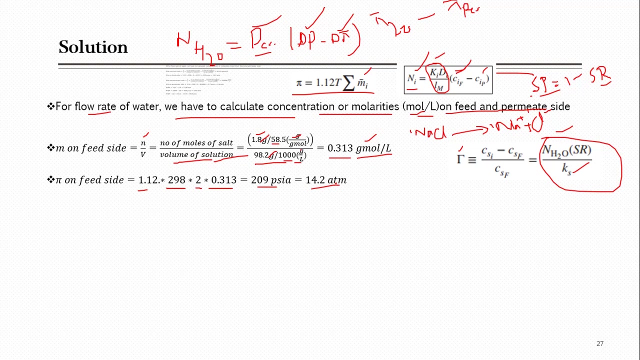 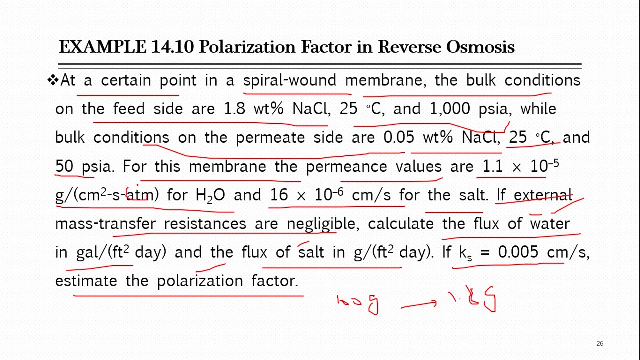 and, as you know, that temperature should be used in Kelvin. So multiply by this 2. 2 indicates like Na plus Cl- These are 2 ions are generated here- and multiply by 0.313 the molarity of 1.. So multiple by 2, because these are 2, and overall you will get it like 209 PSIA. and finally, we have converted it into ATM. why? because there is atmospheric unit somewhere in permeance. here you can observe there was some unit of ATM. 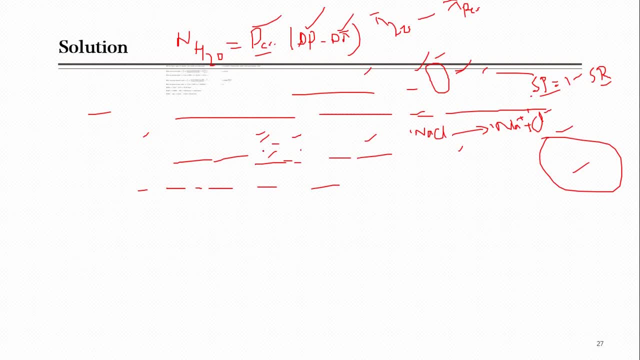 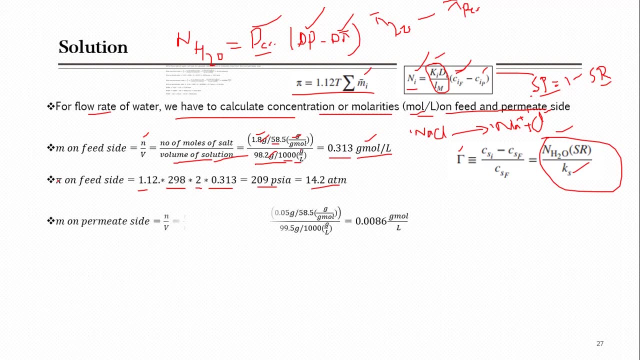 So due to this I have just converted that value from PSIA to ATM. Next same process will be adopted on the permeate side. So on permeate side, number of moles over volume of the solution and number of moles of the salt. again there you have like 0.05 percent salt. that is equal to 0.05 gram if we consider of like 100 gram here. 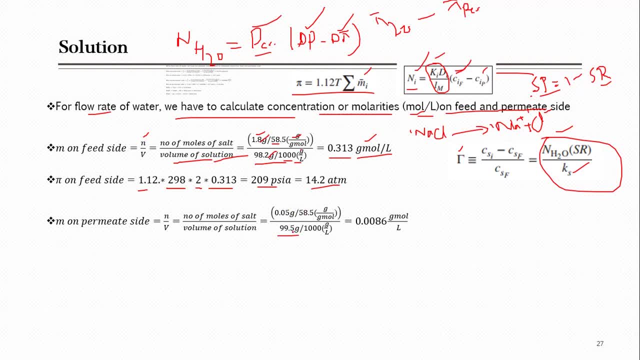 So divided by its molecular weight and similarly then 99.5.. So 99.5 gram over its density, mass over density. that give you the volume. again, here we are ignoring very small amount of salt and we are considering volume of solution is equal to volume of the solvent. 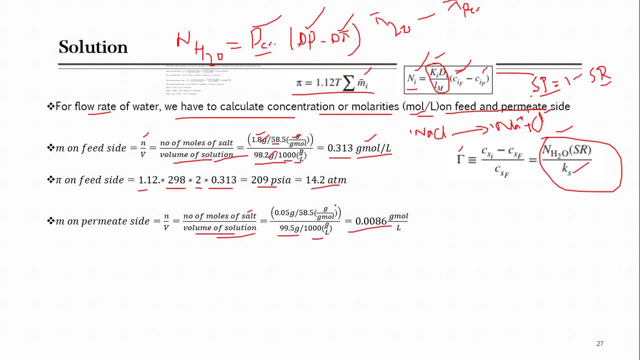 So that is 0.086 gram mole per liter. the same process, and again here again, on this side you have to calculate permeate side pi, because that finally, you have to calculate delta pi. So it will be equal to 1.12 multiplied. 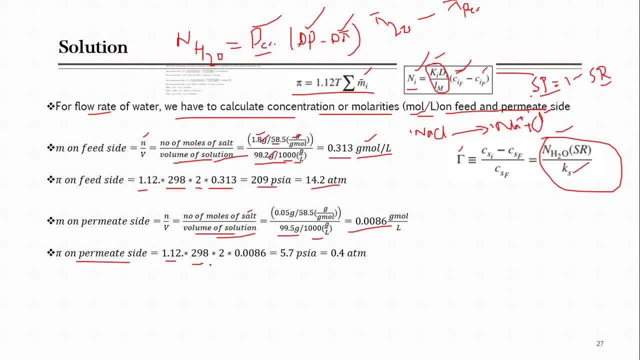 So now this will be equal to 1.12 multiplied. So this is 0.242 by 2.28. this is one energy mass, 2.28 by 2.28. same mean temperature was equal. if you remember from the given data, it was 25 degree c on both ends of membrane or both sides of membrane. 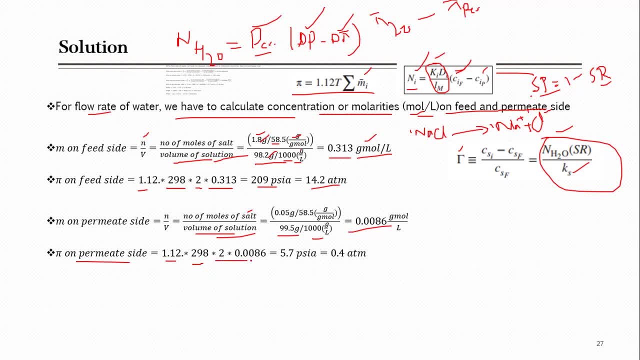 So multiplied again. here NaCl is dissolved into Na and Cl, So it is 2 times, I mean, the smallerity of NaCl. So that is 5.7 PSIA, or equal to 0.4 atmospheric pressure on this mean. 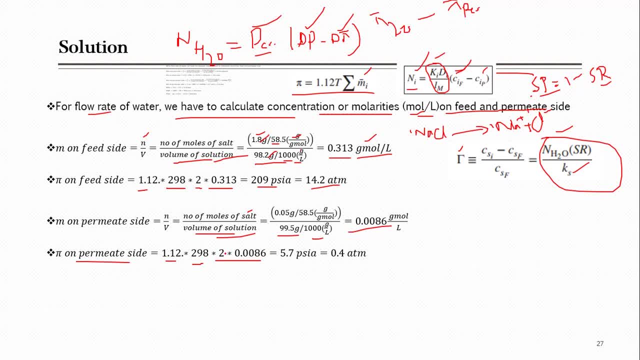 Here one thing: you can observe that osmotic pressure on one side- feed side- because there is very large amount of pressure going to the other side of the membrane. So here, this is the time I am going to add 5.7 PSIA, which is equal to 0.4 atmospheric pressure on this mean. 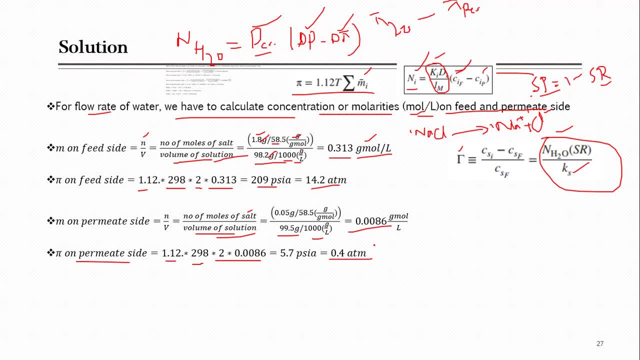 Here one thing: you can observe that osmotic pressure on one side feed side because there is very large amount of pressure. you can observe that osmotic pressure on one side feed side because there is very large amount of salt, So it is higher. as compared to this, on this side it is very low. So if it was suppose pure 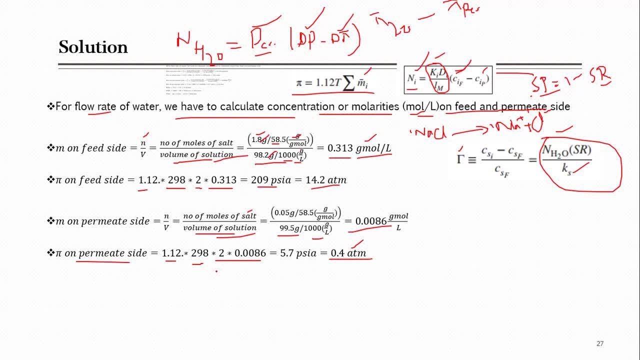 water, there was no salt, so it should be definitely 0. we do not need to calculate this Now, as you have pi on feed side as well as pi on permeate side, so you can calculate delta pi by using these two values, 14.2 and 0.4 atm, and it is 13.8 atm. So then, in this equation, another unknown left is: 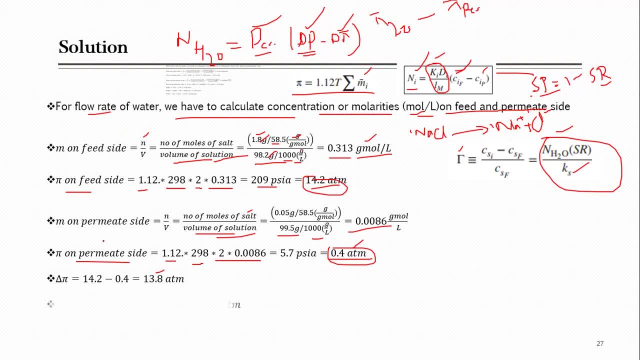 delta pi. even you can calculate that before starting this. but here I have calculated delta pi, so that is equal to 1000 minus 50 and that is equal to 950 psi, and also convert it into atm so that we have all same units. Now, up to here, you have all unknown for this equation. you have 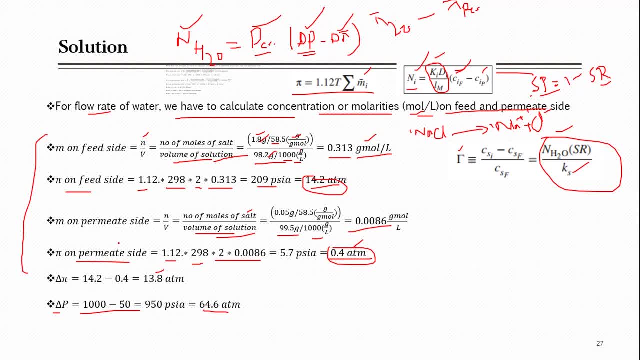 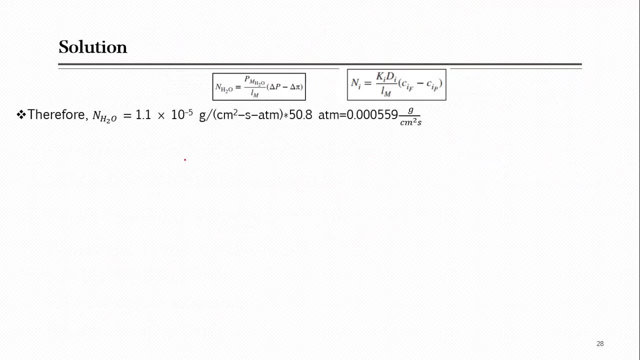 calculated. The main calculation was related to pi. calculation of pi you have done as well, as you have delta pi and permeance was given to you in the main question, So you can calculate flux of water. and for this flux of water we will have like the same equation. I mean this first one, flux of water. 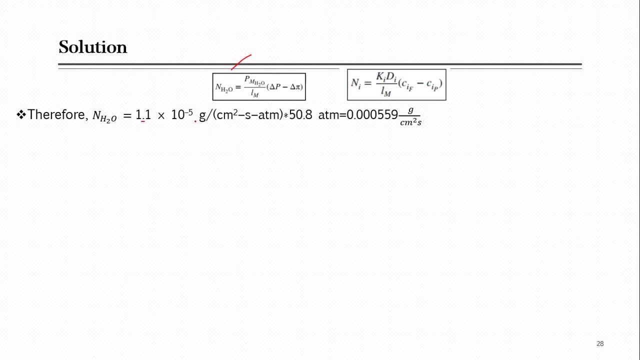 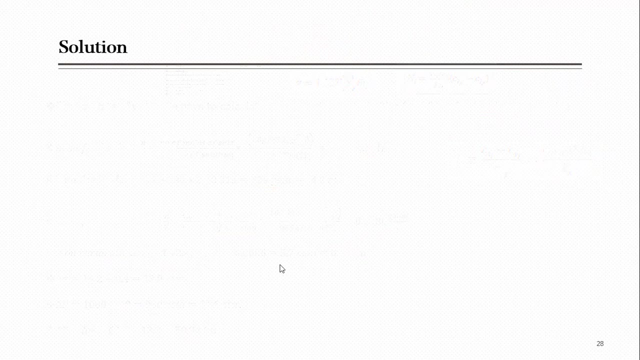 so flux of water here will be equal to permeance, this factor, permeance multiplied by delta pi minus delta pi. and in the last slide, at the last step, We have calculated this delta p minus delta pi and that is equal to 50.8 atm atmospheric. So, based on 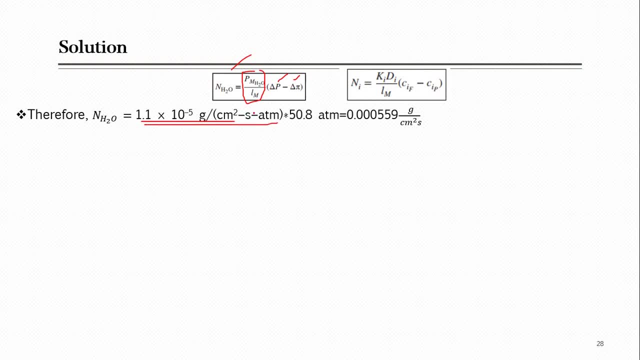 this you can see here that was in gram per centimeter square per second per atm, and multiply by this 50.8 atm. So here what will cancel is atmospheric, with atmospheric because this is on the denominator side and this is on denominator side, so your unit left over are gram per centimeter. 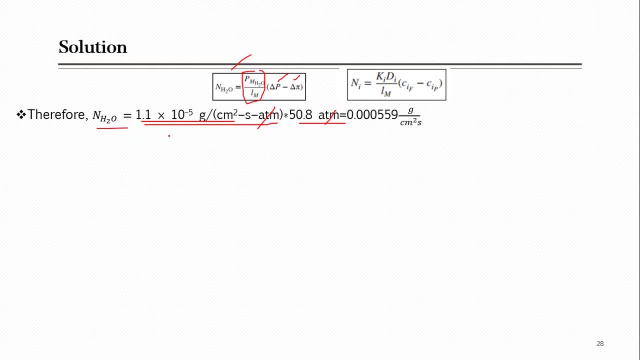 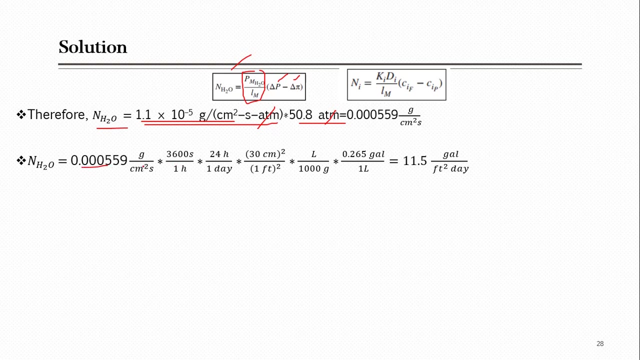 square per second. So this is flux of water through this membrane. Is it okay? Yes, somehow okay. but in the question he has asked us to calculate this flux in gallon per feet square per day. So let us do that conversion quickly. So this is gram per centimeter per second. 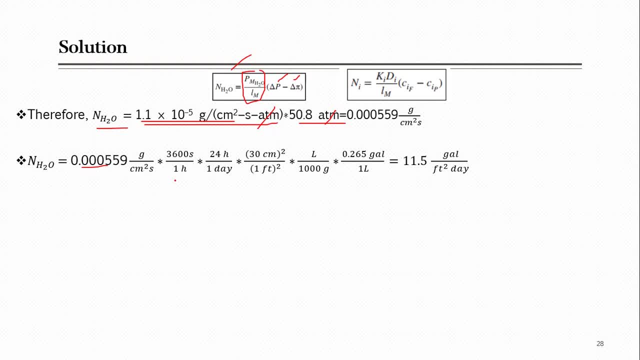 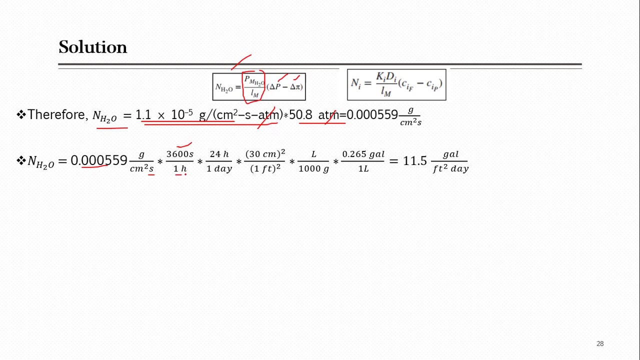 So here I have done clearly for you again in the book it is in the confused form, So just follow one by one. this is second, so let us convert it to day, because our requirement is day for this unit, time unit. So here you have to calculate. So 30 600 second and one hour, so you can use this. one hour mean against 24 hours per day. 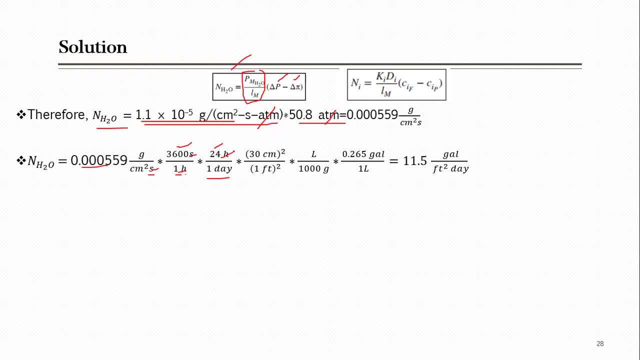 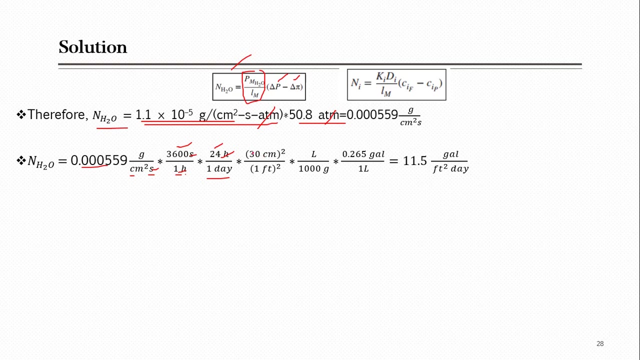 So here, this second will cancel with the second and hour will cancel with r and your units of time are left over. are day Overall. up to here, units are gram per centimeter square per day. Now next unit which need to be calculated are converted centimeter and 30 point something is. it is usually 30 point something, So I have used here 30 centimeter equal to one. 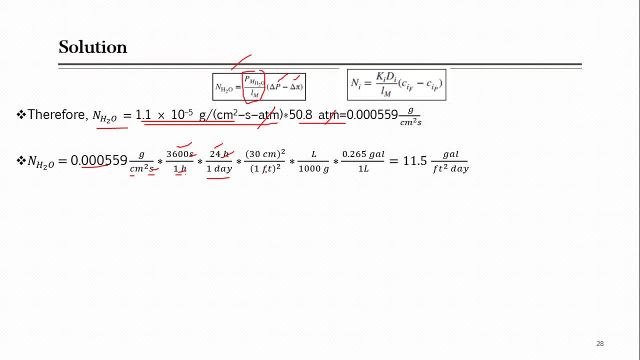 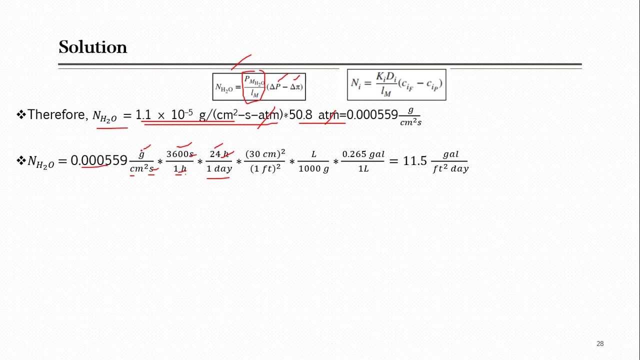 feet and it is square. So on both sides- both side- you will take square. so this will get converted. ah, multiply by now, last part. that is like gram and you have to calculate or convert it to gallon, and this is water. you know, this is unit of mass and you have to convert this to the gallon. that is the unit of volume. so what you have, 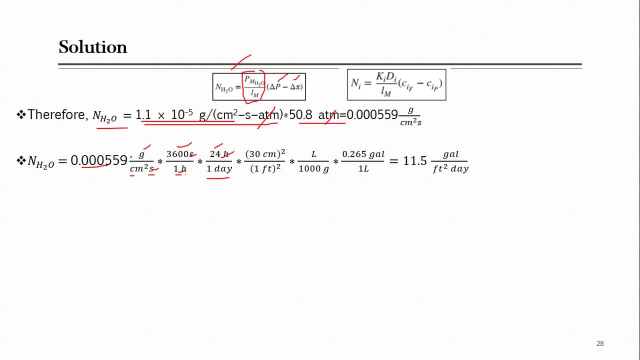 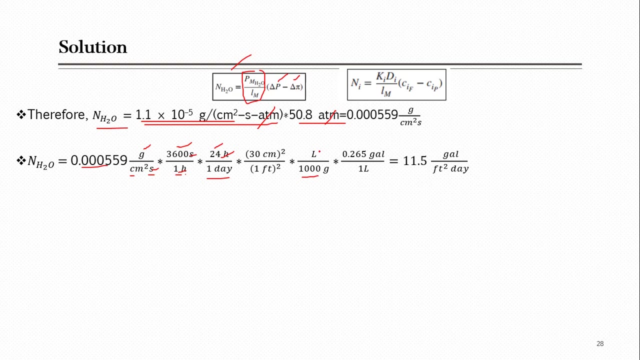 to do? to convert all this equation to the unit of volume, you have to divide this by the density and you can just use this thousand gram per liter. so, by the way, here i have used journal value of thousand gram per liter. but if you want to go more accurate you can look at the like density of water. 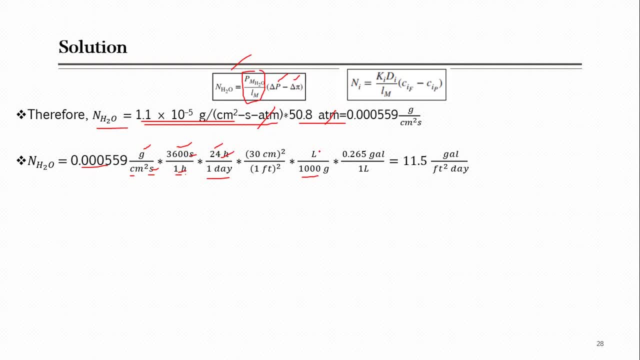 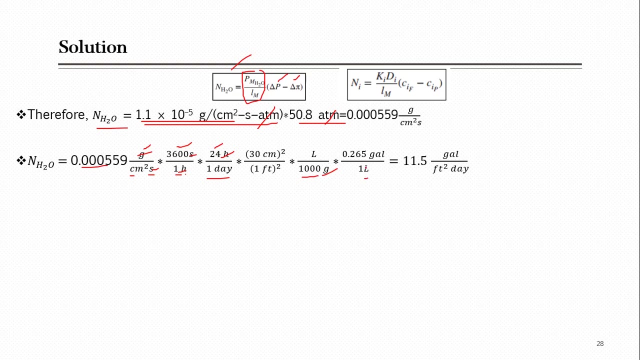 at the given temperature, 25 degree c, i think it should it, it will be like close to thousand again. exactly, not even exactly it will be close, but that that can be used. so here gram will cancel with the gram. and now your units are in the liter, but liter can be easily converted to the gallon, because one liter 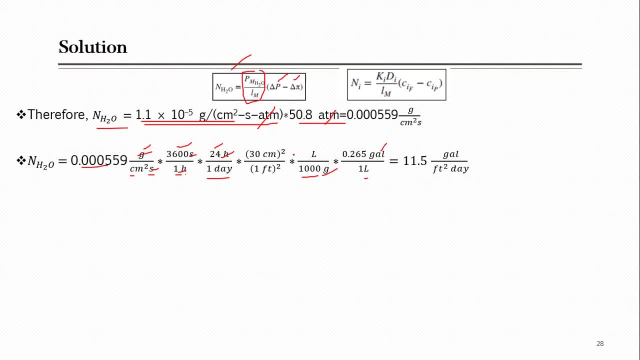 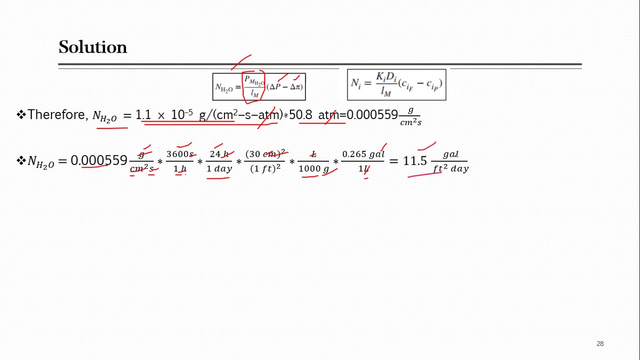 is equal to 0.265 gallon. so with this, overall liter is also cancelled, and now your units of centimeter square were already cancelled. overall units left over are like gallon per day per feet square, and that is 11.5 gallon per day per feet square. this is the flux of water. 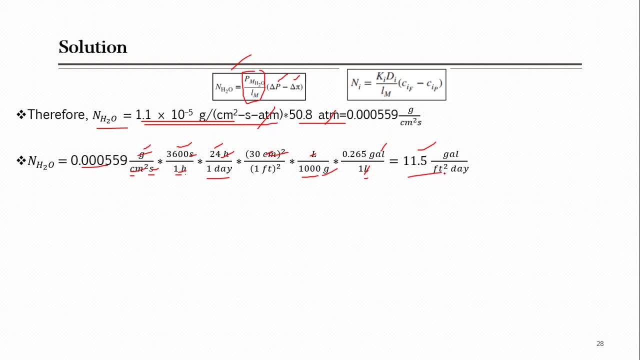 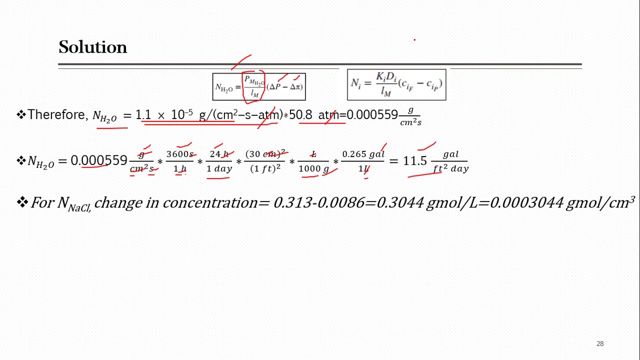 up to here. hopefully you are clear. this is straightforward. just involve a lot of calculation of this unit conversion. so next is actually salt flux. so salt flux can be calculated by using this formula. just look at this formula overall. if- as again i am repeating same- this is permeance, so permeance value of 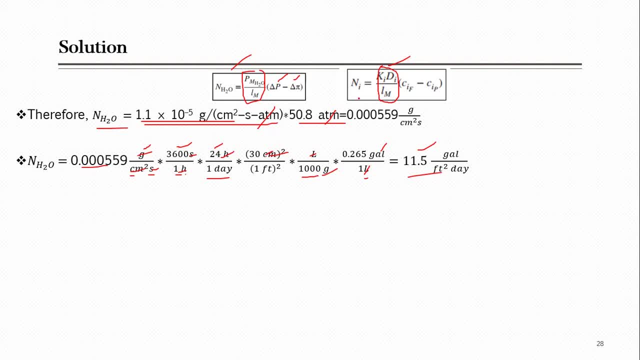 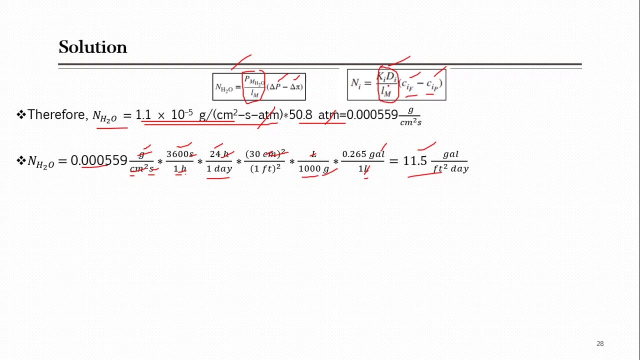 salt NaCl was given. so here Ni it indicates NaCl. so this permeance is given. and their concentration on the both sides, feed side and permeate side. do we have these concentration? yes, in the form of molarity. you have already calculated and here for this mean your value is. 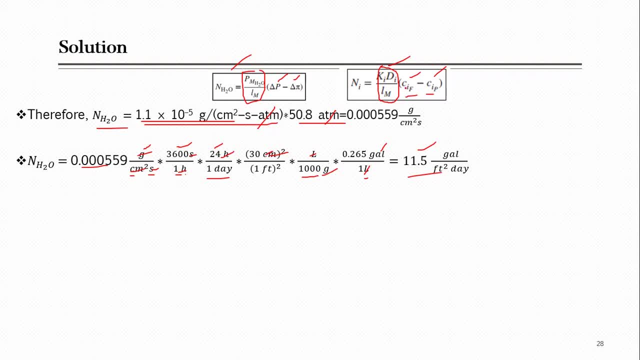 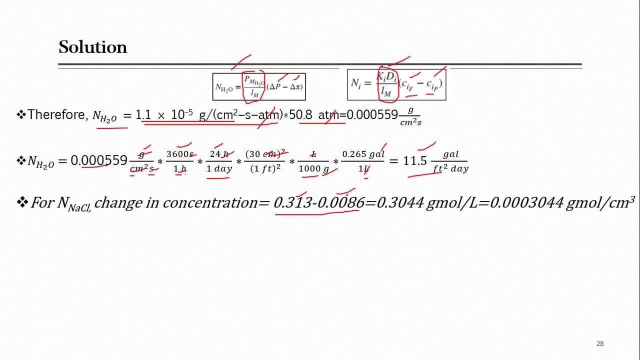 given of permeance in centimeter per second. but this concentration which we have already calculated and that was in the units of mole per liter, so let us use those and make its mean difference. so this was in gram mole per liter, feed side and permeate side. 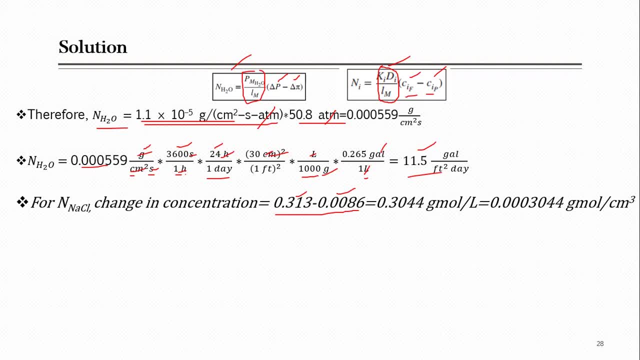 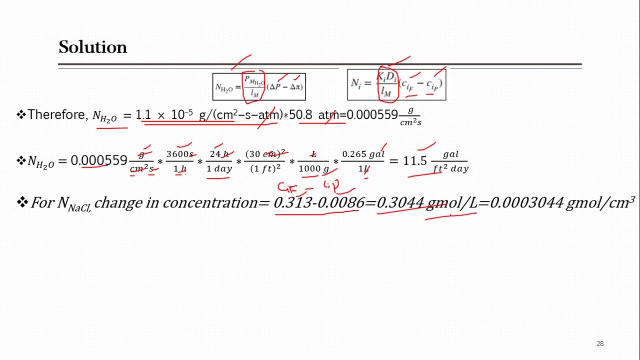 and it will not be related to collapse value, and so that is. is that the value we arePaul pass cross ratio of the N Hit for NaCl change in this concentration. Amcalculating this Cif-Cip, this is calculated HllCif-Cip, so this is ohm condition. so this is 0.310 and 0.00860iq, cal 0086, which we calculated on last slide, so it will be .3044 kalms per later, But we have to convert it. 100.00. этуundes of permeance of NaCl was given in audience of theusion period, so let us talk about p, like her, and infinity, but not only of cative but per moment number, because u know that the units of permeance of NaCl were given in duration of★. 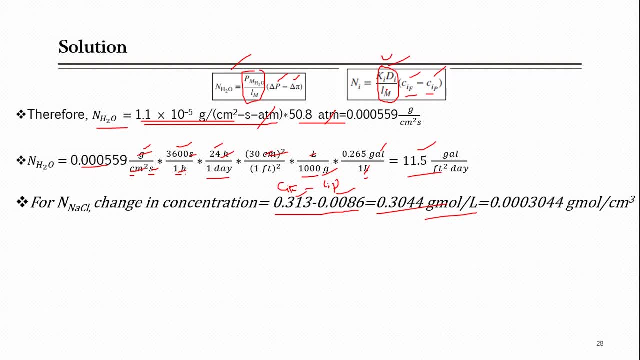 permeance of NaCl were given in centimeter per second. So due to this reason I have just made one conversion from liter to cubic centimeter and this is actually one liter against 1000 cubic centimeter. So when you have to mean cancel this unit it will be like one liter on numerator side. 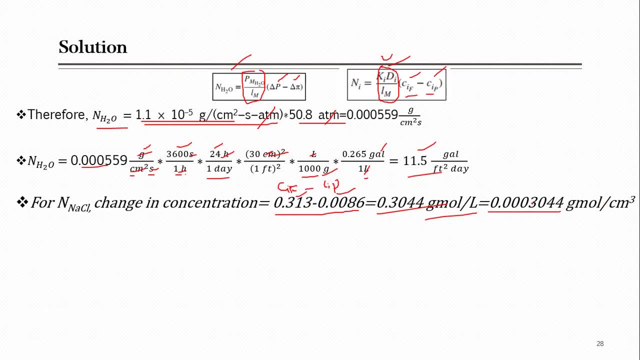 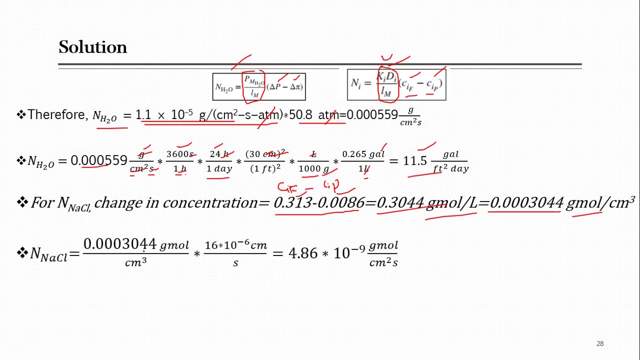 divided by 1000 cubic centimeter- and due to this reason you will get this answer further mean reduced, it is 0.003, sorry, 0.003044- gram mole per cubic centimeter. Now just use this to mean calculate flux of salt by using this equation. this is value of concentration which you have. 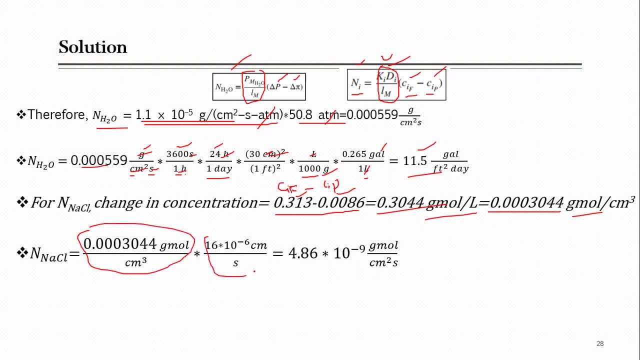 just converted in the last step, multiply by its permeance, that is 16 into 10 to the minus 6 centimeter per second. So overall, if you cancel the unit here, centimeter will cancel with this and what you will left over that is gram mole per centimeter square per second. and this is 4.86 into 10 to the minus 9. 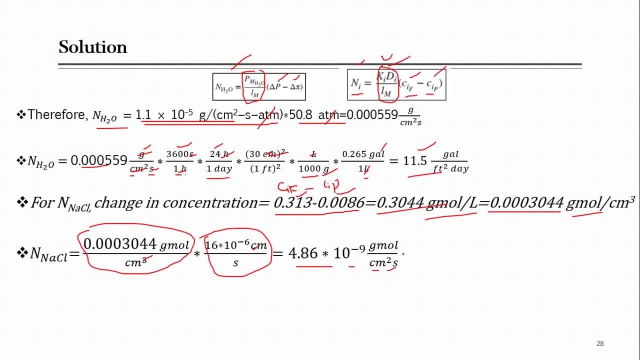 gram mole per centimeter square per second. If you remember, he asked us to calculate this in gram per feet square per second. So again we will make here unit conversion. So just start with the first, easiest one. again mean this second is converted in today by using these two time. 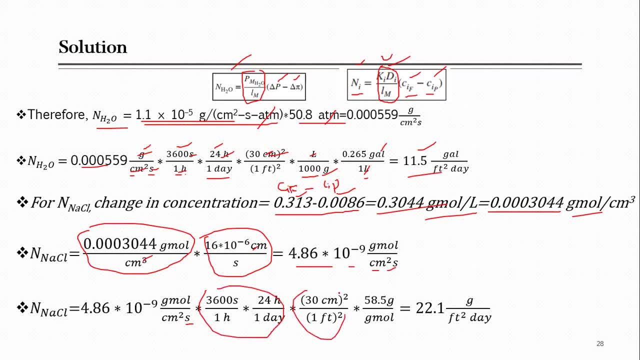 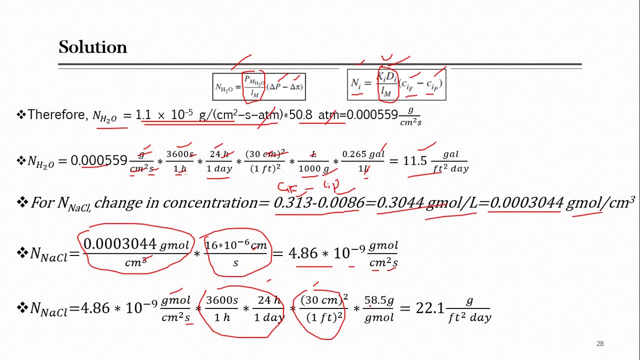 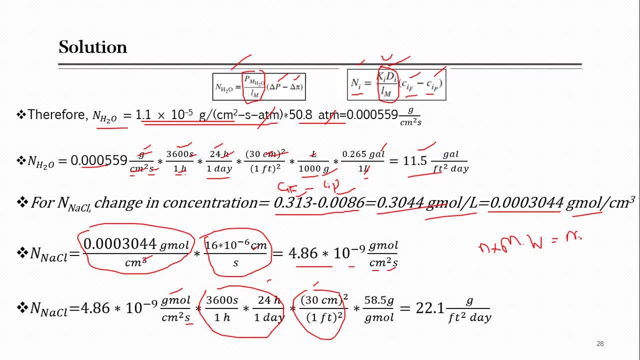 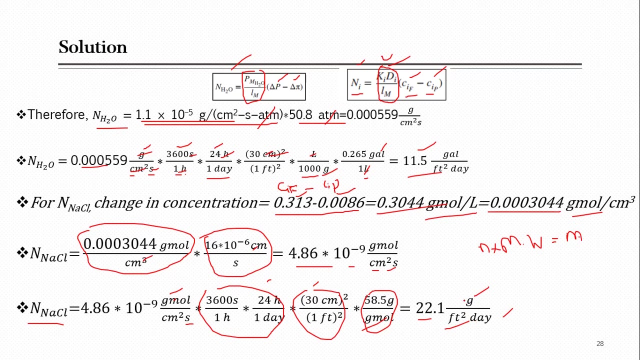 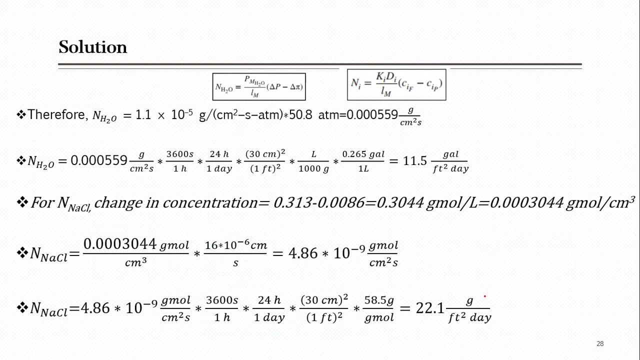 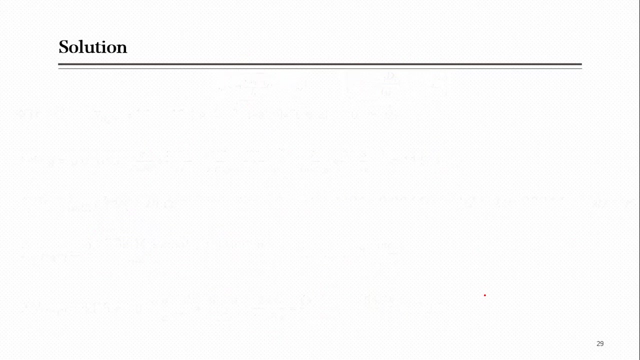 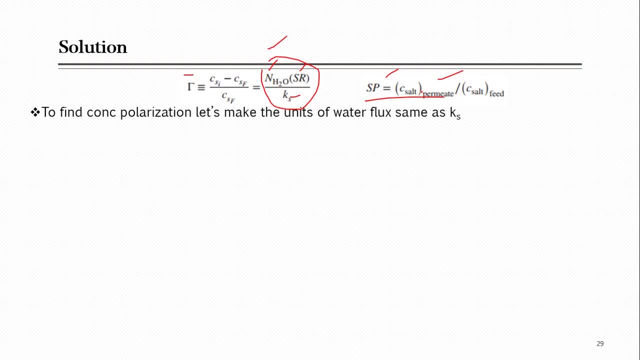 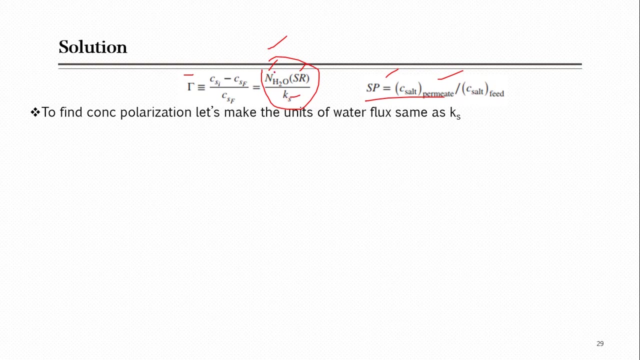 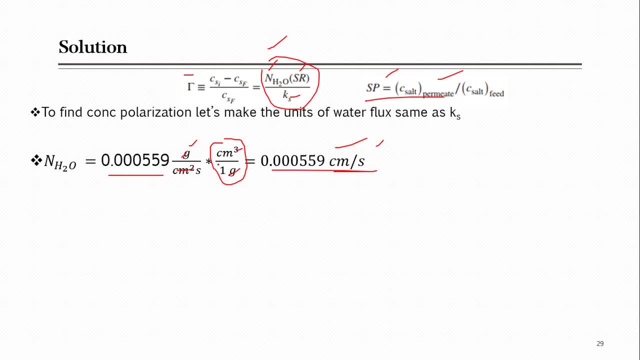 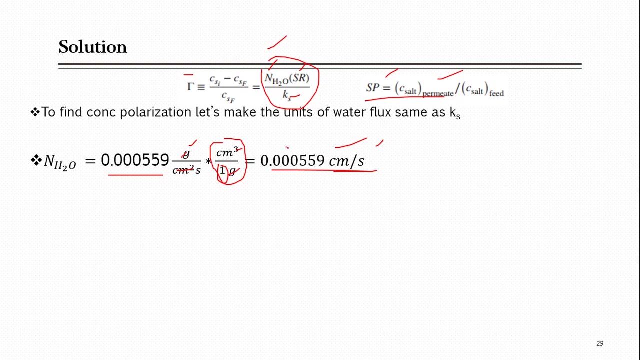 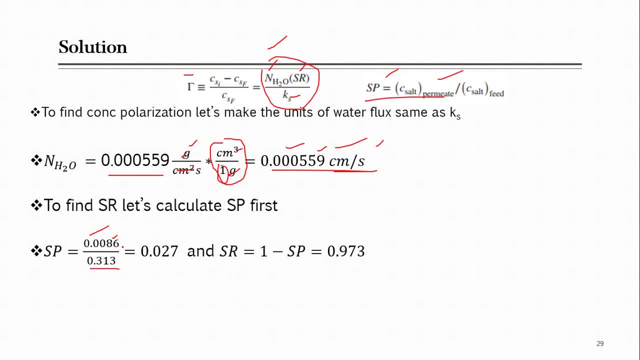 salt on permeate side over concentration of salt on feed side. So this already you have for mean, any unit you can pick, because unit will cancel and finally its value is 0.027 here and with this you can calculate SR and that is value is 0.973.. It is mean 97.3 percent. 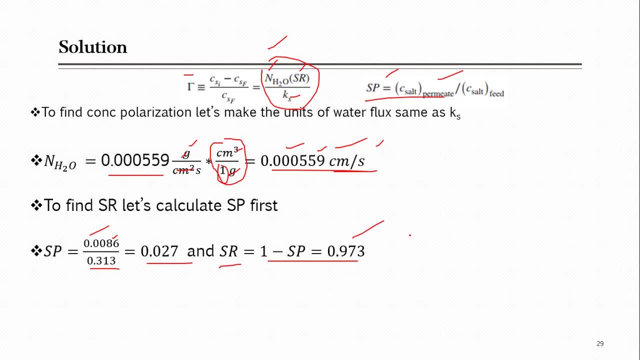 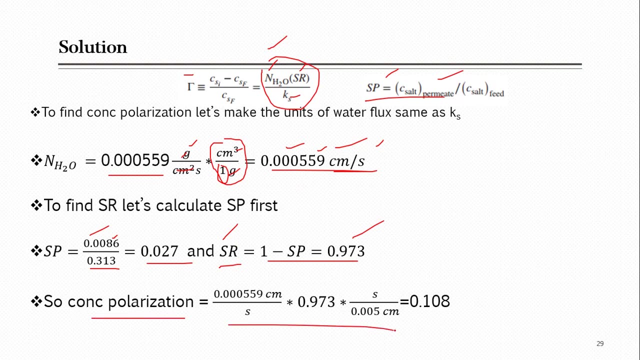 salt is rejected only mean 2.7 percent salt has passed through this membrane. When you have all these parameter now- Ks was given in the question- flux of water is converted to the same unit and salt rejection is calculated. So concentration polarization is easily calculated. 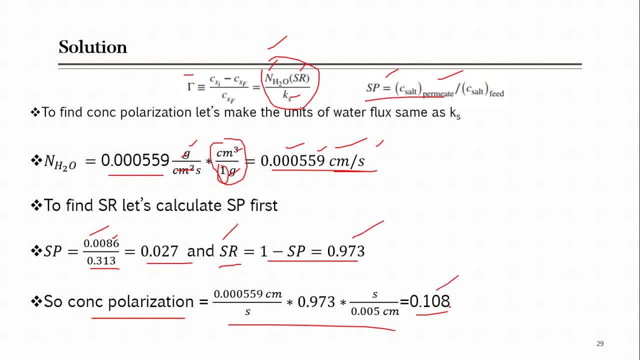 and that is unit less parameter, and its value is 0.108 for your case. for your question, So that is the value. if you remember, for concentration polarization he said that if value is greater than 0.2 then there is a problem, then you have to change the membrane.